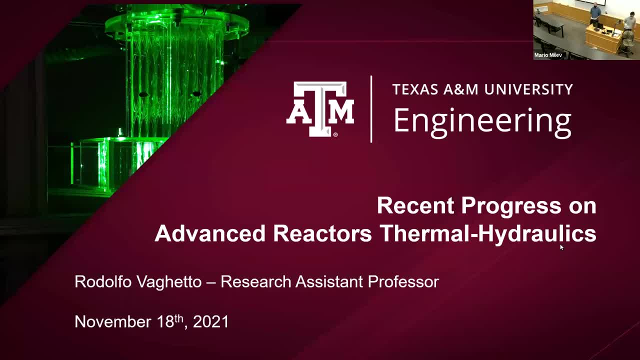 Welcome everybody to this week's department seminar. As always, just a quick few ground rules. If you're not speaking, please mute your microphone And then, whenever we go to the Q&A, you will have the option of either raising your hand to ask a question or you. 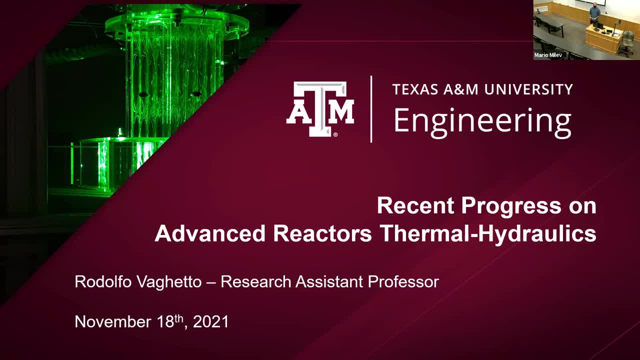 can type it into the chat and then I will read it to our speaker today. So, whichever one you feel better with, Let's see here. Department announcements. I don't think there are. I think this is the last one, right? So this is our last seminar of the semester. 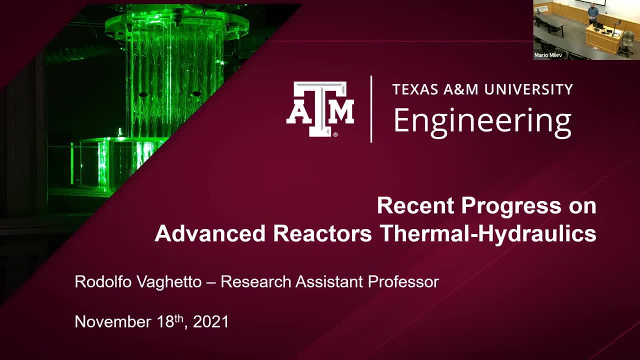 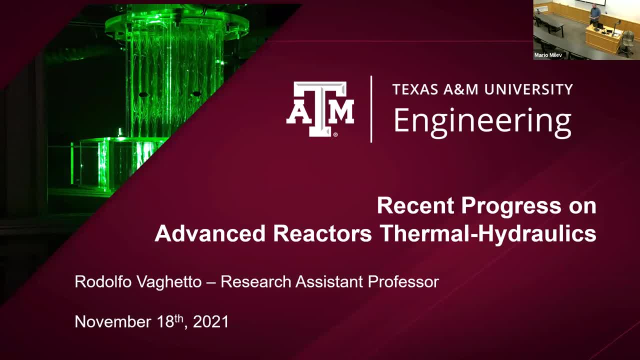 is the last one, So this is the last one, So this is the last one, So this is the last. Dr Viguetto was part of a challenge project that led to the resolution of one of the most complex generic safety issues for light water reactors in history, the GSI-191, resulting 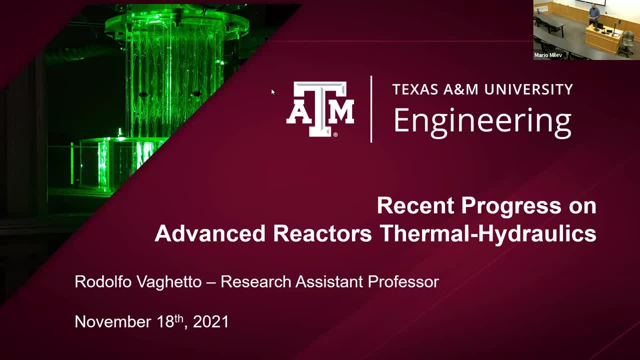 through an innovative methodology that has been accepted by the regulator and referenced by several utilities nationwide. With that, I hand the floor over to Dr Viguetto, and thank you for being here, sir. Yes, thank you so much, and I really thank everyone for inviting me to speak today at 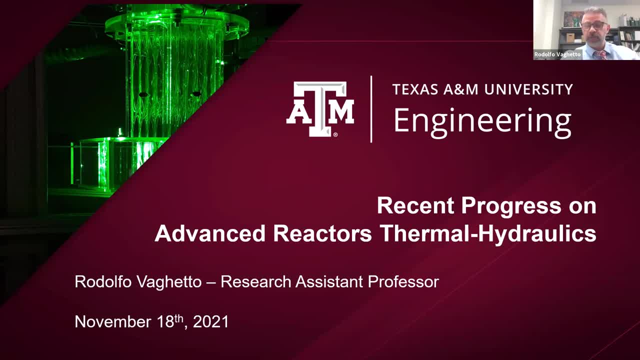 your last department seminar of the semester and I thank everyone joining the seminar today for staying with me for the next hour. I am particularly happy to present today And the reason is because I'm very happy to be here And the reason is because the Thermodralic Research Laboratory, where I work and conduct 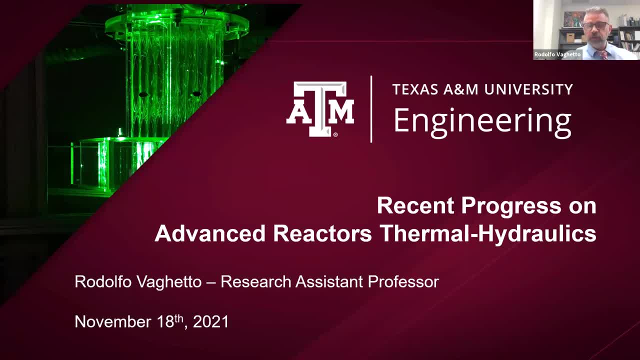 research is strongly connected with several of the professors and researchers at your department, And approximately one year ago we have established a new project that is led by Professor Avramova and Dr David Holler and that involves the use of some of the experimental datasets that 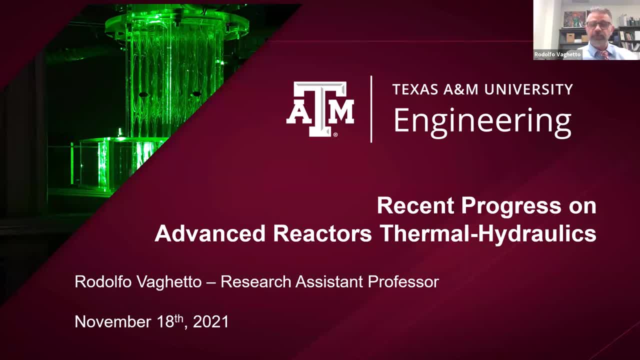 we have produced from the 60s And that is the 21-pin wire wrapped fuel bundle replica, which is actually the core of the discussion today. So, before I go through my presentation, I wanted to give you- I prepared a very quick 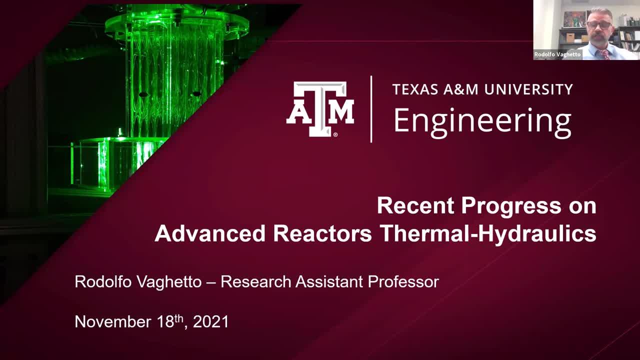 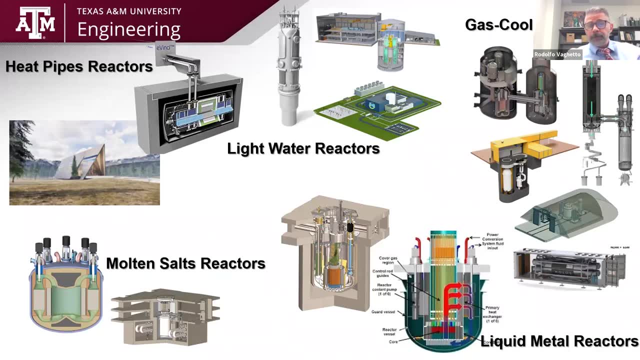 overview of the current reactor technologies that are available in the United States. Okay, So this is an overview of the majority of the nuclear reactor technologies that are available in the United States, And I'm going to start by talking about some of the reactor design and technology currently. 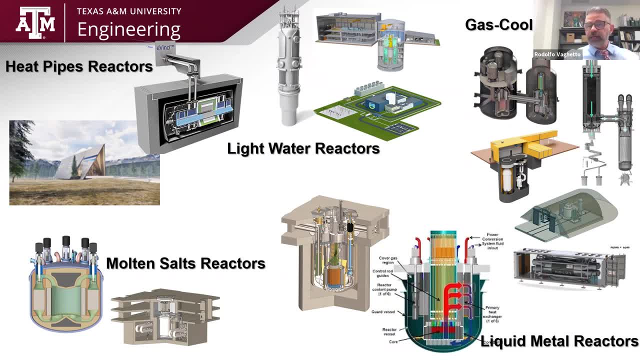 under consideration. I divided by reactor technology And, if we start from the top, I selected some reactor vendors that are currently considering to reuse some of the technology available, especially the one coming from the large light water reactor currently in operation, And by doing that, they have somehow overcome some of the challenges that we have faced. 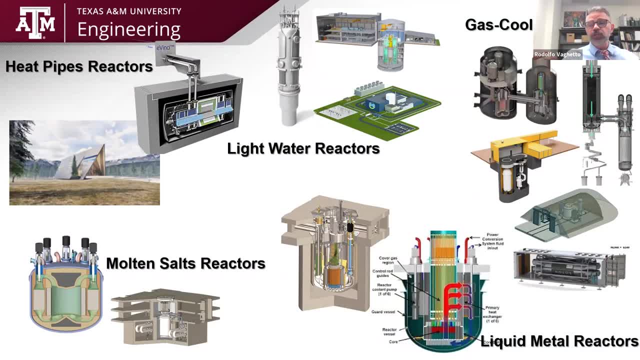 in the last few years And I'm going to start by talking about some of the challenges that are related to the use of brand new technology of coolant. Still, there are some challenges here because the design, operating conditions, certain geometrical parameters are different and requires special attention and additional research and development. 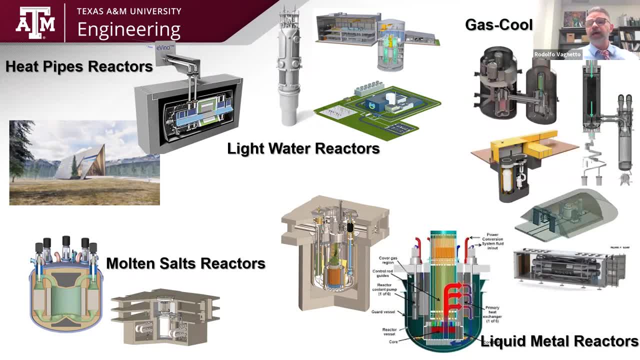 If we move clockwise on this slide, we go toward the technologies and coolants that we are currently using. And if we start from the top, I selected some of the technologies that are currently under consideration. And if we start from the top, I selected some of the technologies and coolants that we are. 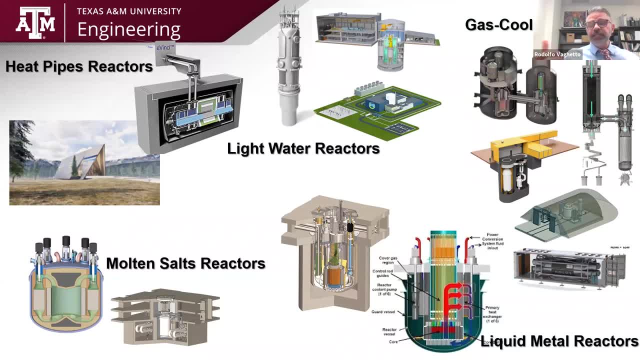 currently using that have been less and less explored. So, gas-cooled reactor: to be honest, they have been around for quite a bit. They have been a gas-cooled reactor in operation. There are new gas-cooled reactor went online recently in China. 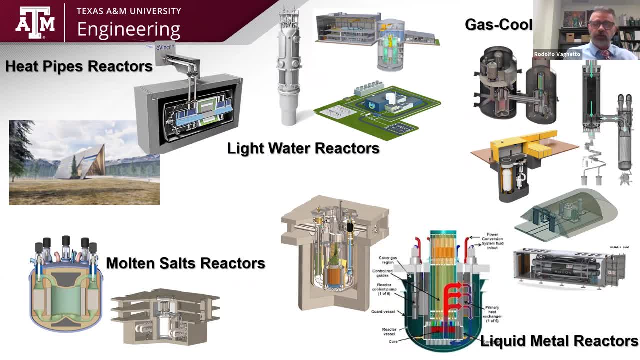 So the use of gas as coolant is not really a new idea. but the new ideas here that pose challenges to the core developers, to the reactor developers, is the different type of core designs. There are technology: they are using pebble bed designs. 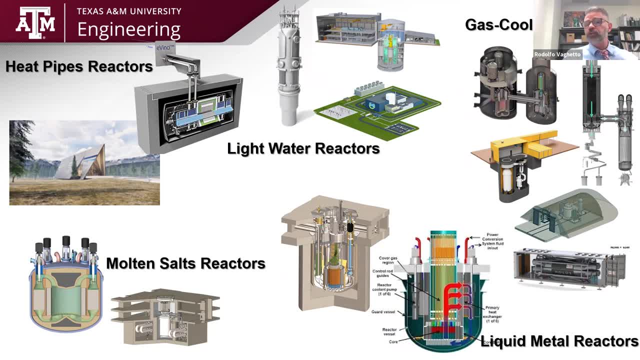 technologies. they are considering graphite block, some other designs that they are still considering fuel rods in their core. So again, there is a very active research and development that needs to be accomplished before increasingly increasing the maturity level of this technology to be deployed for energy production. 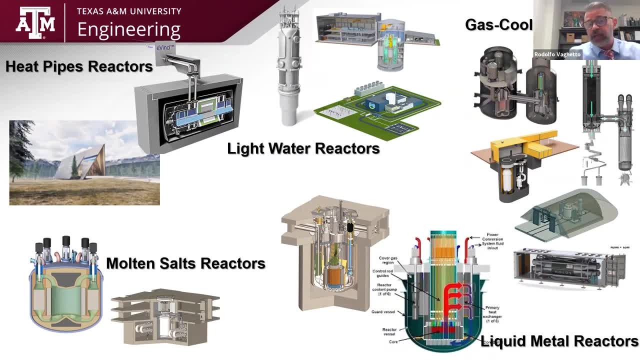 And if we move forward to liquid metal fast reactor again, they are not relatively new but not very old And because of the challenges related to the use of liquid metal as coolant and the challenges related to the geometry of the core, have motivated a really wide range of experimental 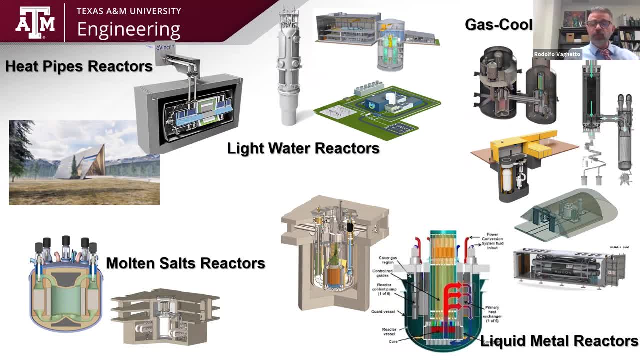 and computational activity worldwide. So if we move to the molten salt reactor and the heat pipe micro reactor now, we are moving towards technology that are relatively new, where experimental data are really relatively limited if compared to the ones available for light water, gas-cooled and liquid metal. 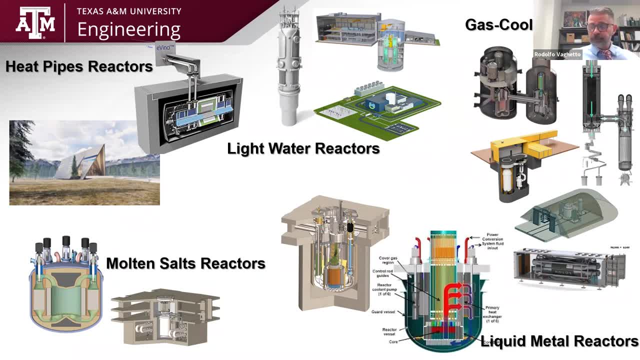 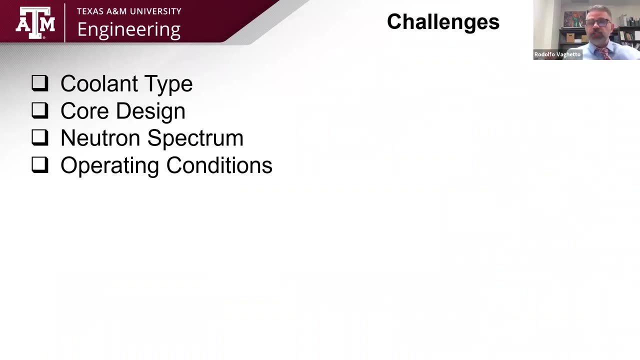 And here challenges are even more interesting, so to speak, And that's where the market is. The majority of the research and the development at the moment is focused. All these reactor designs, they share some challenges And the challenges are related to the choice. 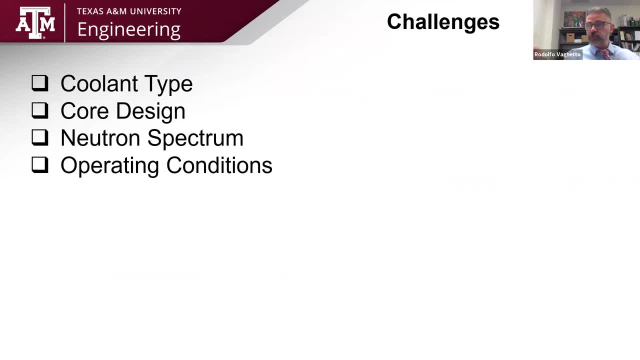 of the coolant type, the core design. I mentioned pebble bed road bundles or graphite blocks design. They are related to the choice of the neutron spectrum rather than the isothermal or fast, and the And are finally related to their operating conditions. 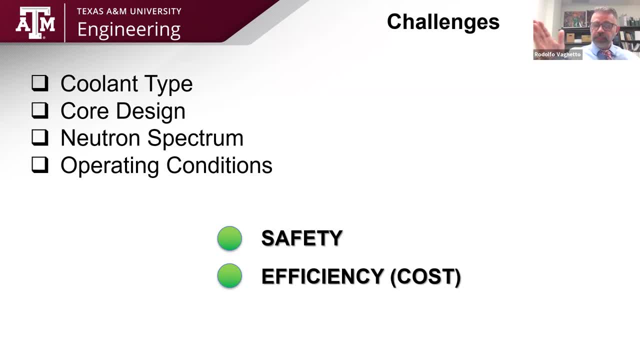 So then, why a reactor design may choose one option or another, or a combination of these options. Well, the reactor designers are currently working all toward making sure that we have the best source of electricity, And the second one is efficiency, So making sure that the operational costs 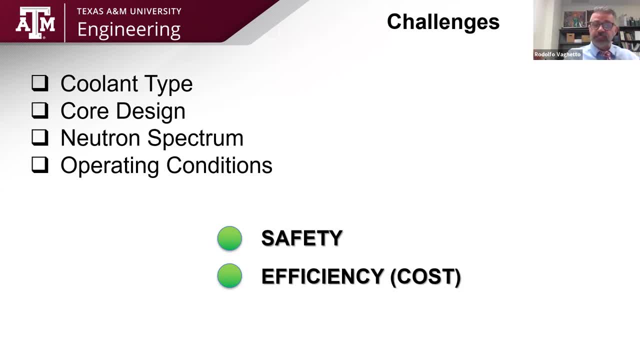 are actually minimized so that that specific technology can be as competitive as any other clean energy sources available today. So our goal and our work that we are all doing as researchers is to make sure that we we maintain high level of safety and reduce the operational costs. 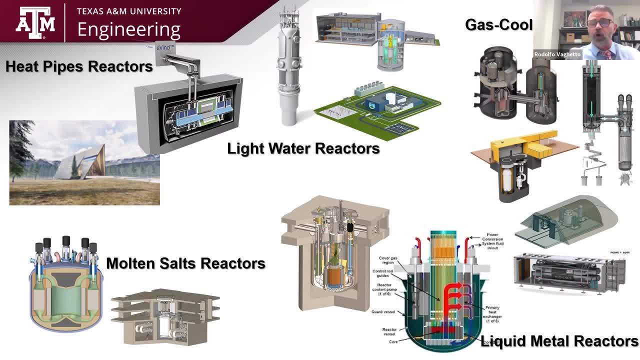 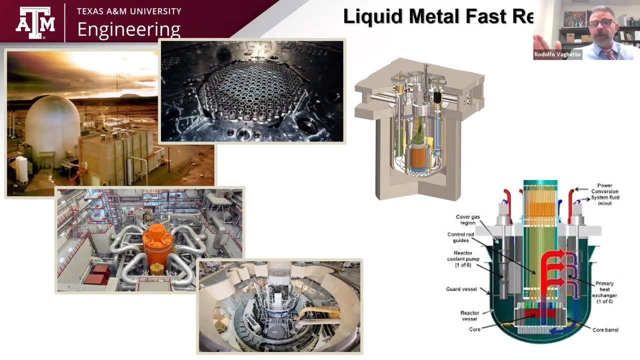 Now, if I go back to this cartoon where I showed all the reactor technologies, I decided to select the liquid metal fast reactor that are actually in the middle. So there is a technology that is relatively mature compared to the molten salt and heat pipe reactors. 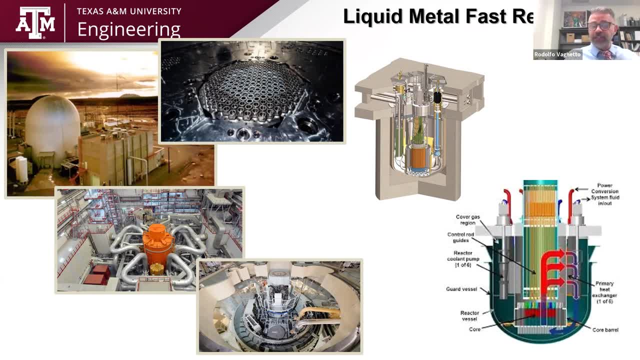 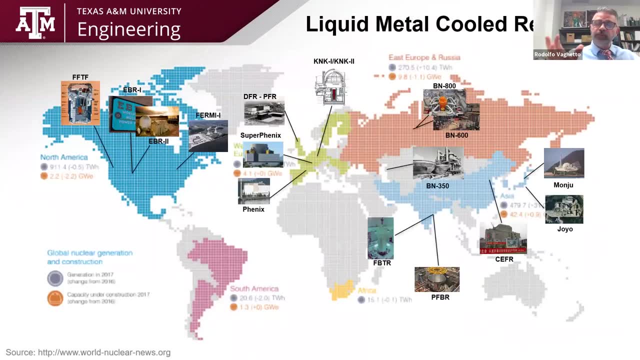 but still requiring, you know, a lot of energy. So I think it's important to understand that you know we are working on very active research and development, If just to give an idea of the amount of activity and research that has been conducted worldwide. 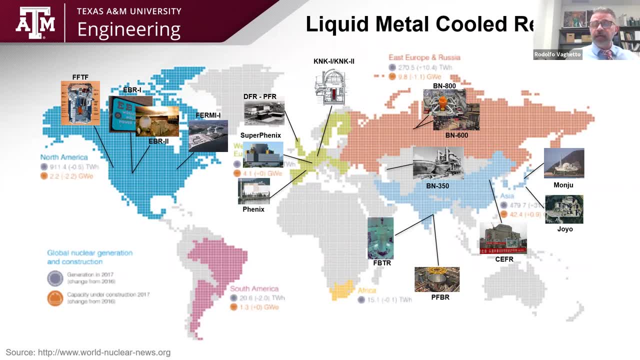 this map shows the location of the liquid metal research reactor that have been designed and operated in the world, And some of these reactor have a large size and they are very, very large And they are very, very large And they are very, very large. 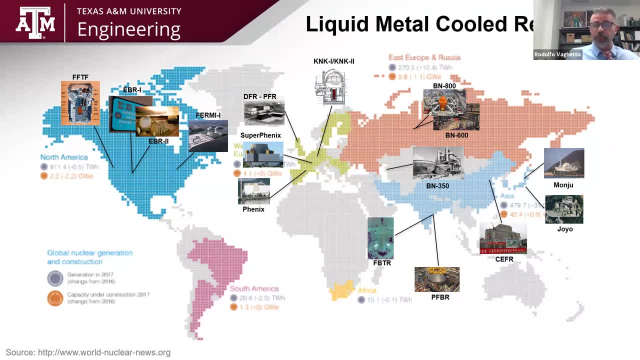 And they are actually power reactor, like the one operating in Russia. And if I would overlap to this map that research and development that universities like North Carolina State University or Texas A&M University, or national and international laboratories entities and industry are currently performing in the area of you know, 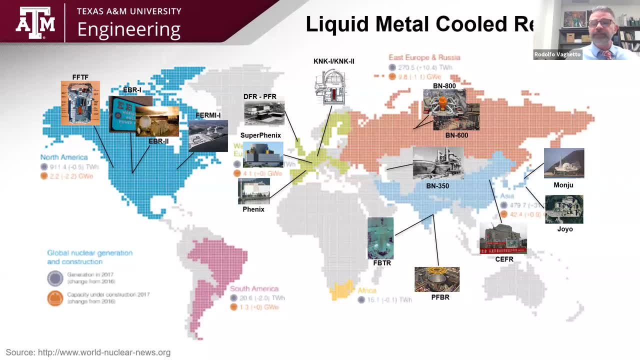 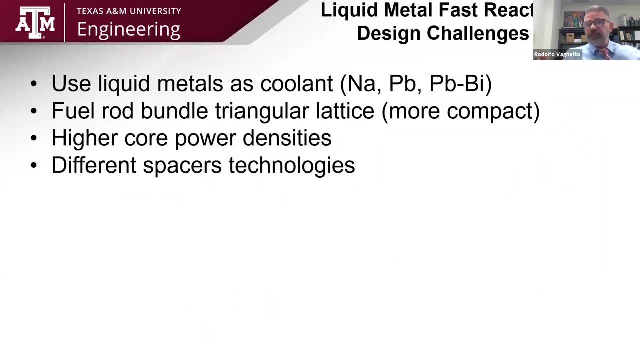 liquid metal fast reactor. this map will be completely covered by small icon and pictures. So the reason why the liquid metal fast reactor are attiring such attention is because there are certain specific design challenges, Not only because they use a liquid metal as a coolant. 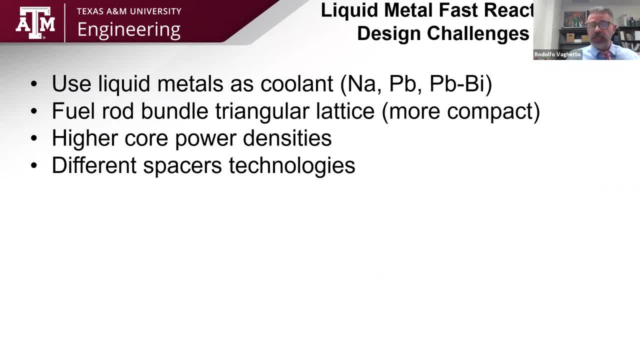 here I mentioned three of the current options that are considered, but because there are certain specific design challenges that are considered, but because there are certain specific design challenges that are considered, but because there are certain specific design challenges and I focus specifically on the core. 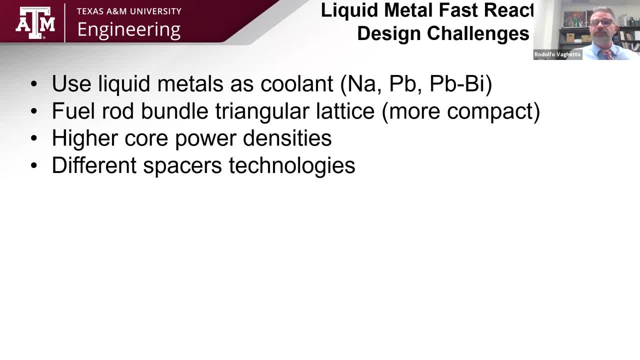 Fuel road bundles in liquid metal fast reactor, just because you don't need to use a moderator. They tend to have a more compact design. They change the lattice of the road from a square lattice, typical of a light-water reactor bundles, to a triangular lattice. 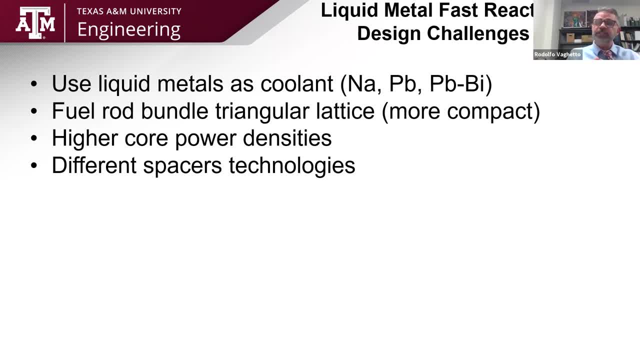 Now, by doing that, you have a more complex thermodralic behavior of the bundle because of the smaller sub-channel flow areas. But you have also other challenges. You have a higher core power densities, So here you need to really understand. 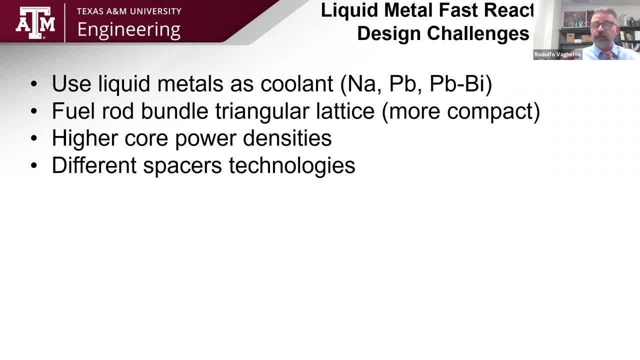 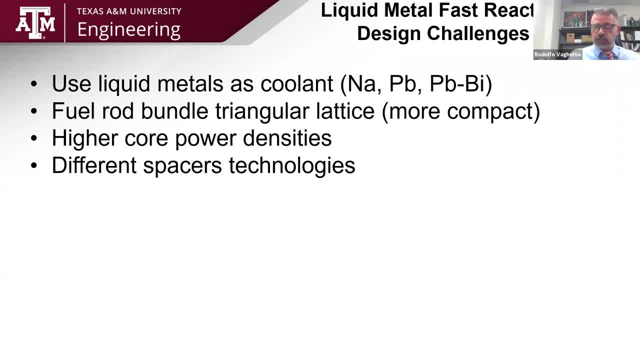 under consideration for the spacers. So spacers in the fuel bundles are used to maintain the lattice during operation. So spacers in the fuel bundles are used to maintain the lattice during operation. So prevent the pin displacement. At the same time reduce the flow-induced vibrations. 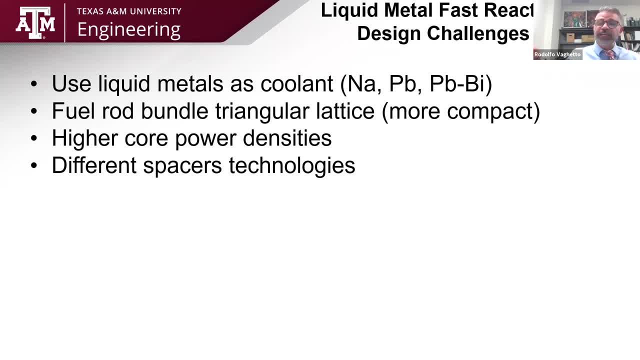 Some spacer grid designs, for example, are meant to increase the heat transfer mechanisms. But every time you try to attempt to improve the heat transfer mechanism, normally there is a drawback, And the drawback is usually the pressure, and the pressure drop through the core. 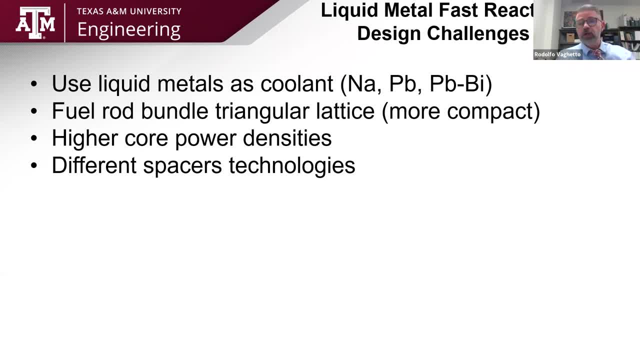 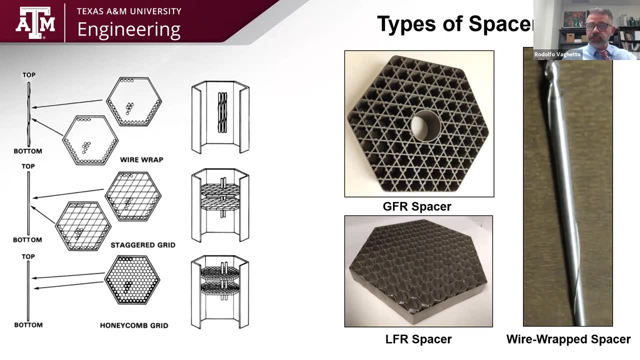 which is an important parameter when you design a reactor, not only for estimating the required pumping power, but also for safety reasons. I collected a selection of pictures of the current spacer technologies that are under consideration for liquid metal fast reactor fuel bundles. The one at the bottom is what is called the honeycomb grid. 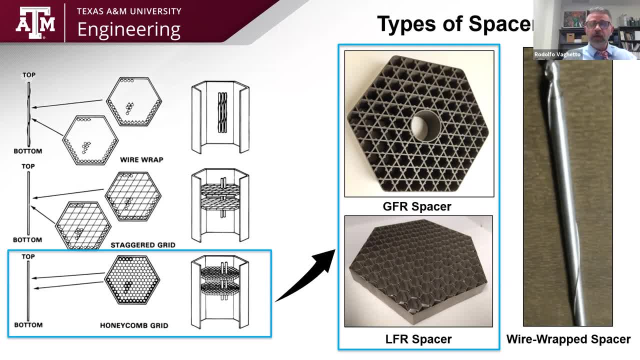 These two pictures are not actually taken from Google, but these pictures are pictures of spacer grids that we are currently investigating in our laboratory And I have it here with me. If you have the camera on, you can see it. This is a typical spacer grid. 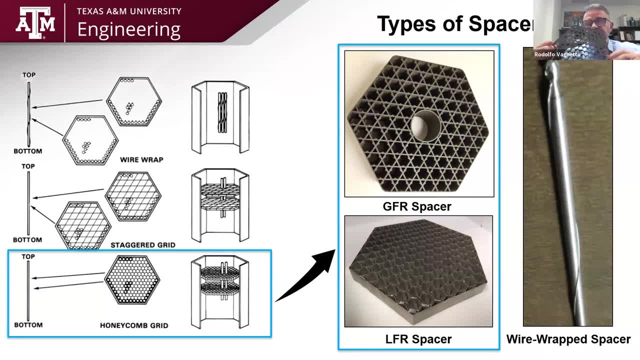 It was 3D printed with the stainless steel 304.. This is a typical spacer grid mounted in a 127-pin liquid metal fast reactor And if you go to the picture at the top, it's another 3D printed spacer grid. 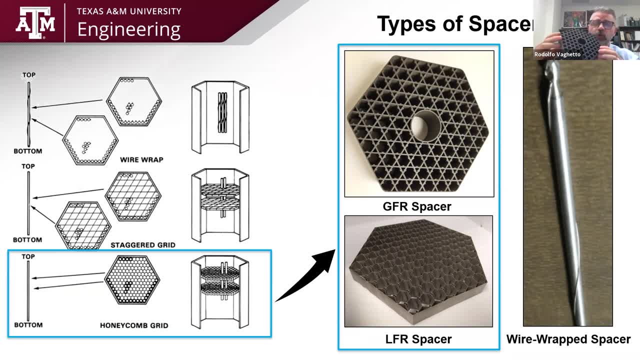 This is used for gas-cooled fast reactor, while the coolant is different. As you can see, the geometry is very similar And this was 3D printed with plastic material. Both the spacer grids are mounted in dedicated fuel assembly replica that we are using to investigate the thermo hydraulic behavior. 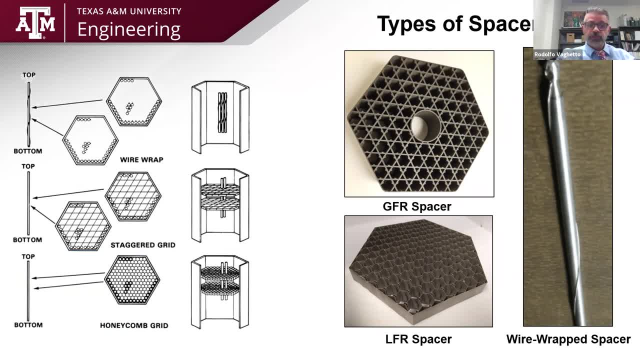 in this reactor core configurations. And there is also another interesting spacer technology that probably most of you are familiar with, and it's the wire-wrapped spacer. This technology consists of using a metal wire. The wire is actually wrapped individually on each pin. 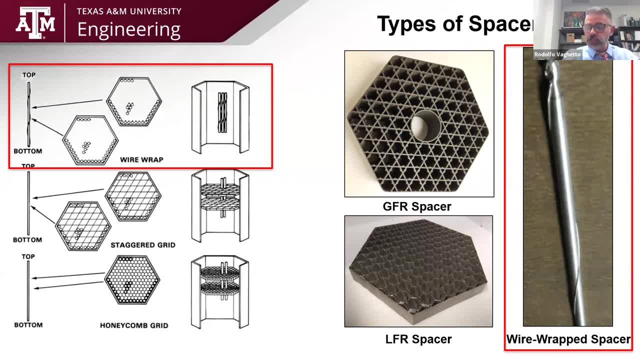 So there are no spacer grids at any axial location in the bundle, but there is instead a continuous spacer that is maintained by the use of this wire. So the wire is a spacer, so it has the same capability of a spacer grid: It maintains the lattice. 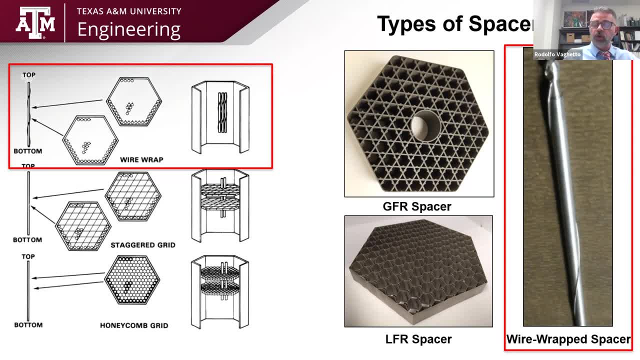 It prevents it, It displaces the pin during operation And it also reduces the flow-induced vibration. But, as you can see, the effect of the wire on the flow and heat transfer has an impact And the thermo hydraulic behavior of these bundles are so complex that it has motivated. 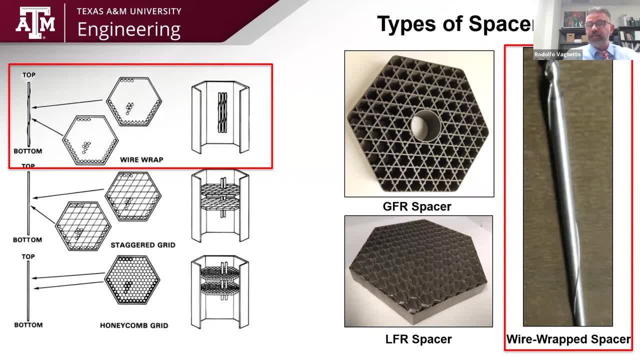 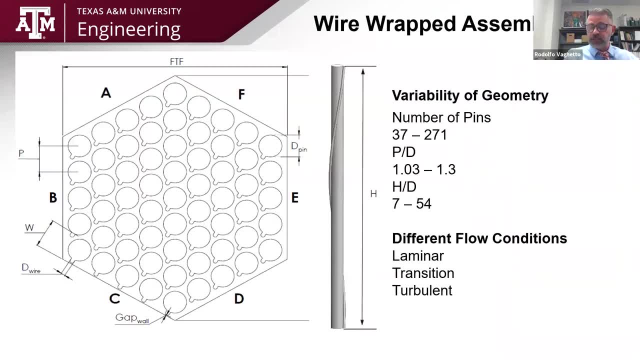 a very wide computational and experimental research worldwide, And that was basically motivated our laboratory, the thermo hydraulic research laboratory, to build the test section that I'm going to show you in a couple of minutes But, before moving, that I wanted to share with you. 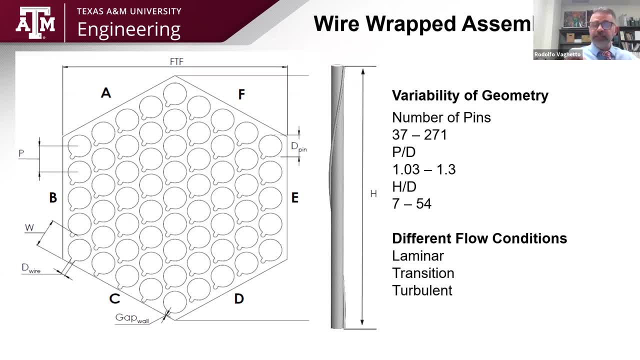 specific challenges when studying the thermo hydraulic behavior of these bundles. There is a very complex geometrical characteristic characteristic of the bundle, So triangular lattice. There is a number of pins that can vary based on the location of the fuel assembly in the core and based on the outer core design needs. 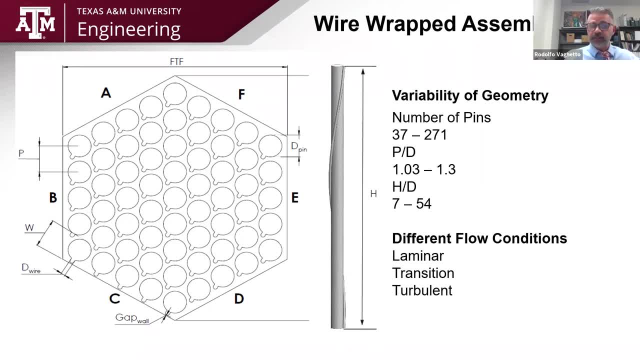 Usually these pins are enclosed in an hexagonal duct, So between the outer ring of the pin and the duct you have a gap. That is usually indicated with the letter W, And this is the edge pitch And the P over D, the pitch over diameter ratio. 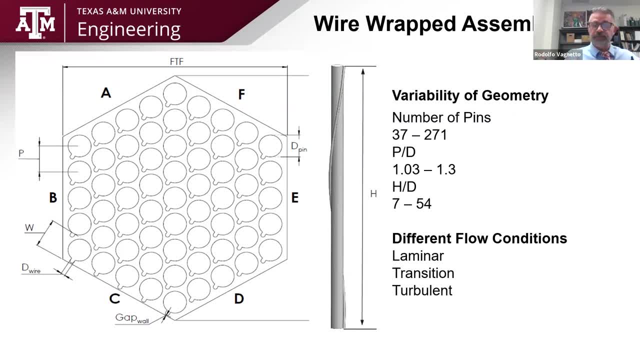 which will give you an idea of how compact is the fuel bundle, And, of course, the helical pitch over diameter ratio, which may vary and will tell you how fine the helical the wire is wrapped around the pin. Of course, during normal operation, 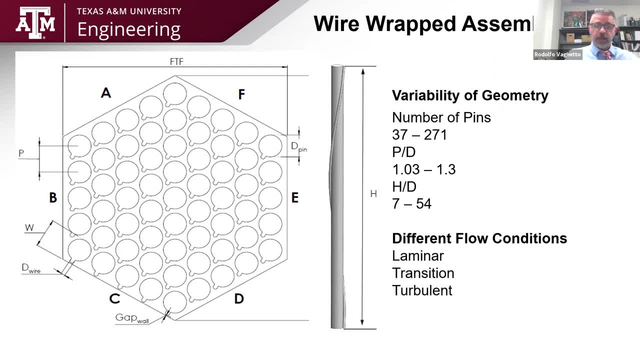 these bundles are supposed to work in the fully turbulent regime But of course during transient scenario, during the accident scenario, you may transition to transition and laminar regimes. So if you combine together all these possibilities, you realize that you really need to have a wide variety. 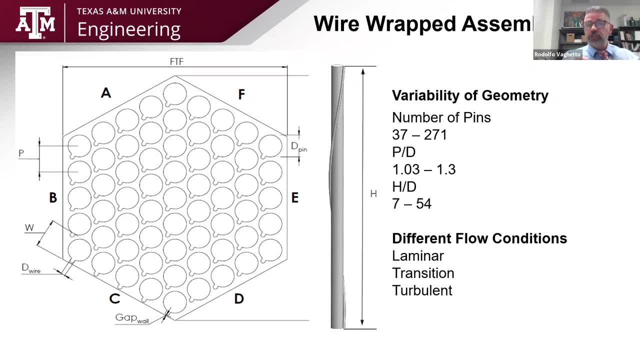 of experimental data points that are important not only because we have to understand better the thermodralic behavior and how each parameter and the combination of these parameters impacted the thermodralic behavior, but also because the experimental data are always important to. 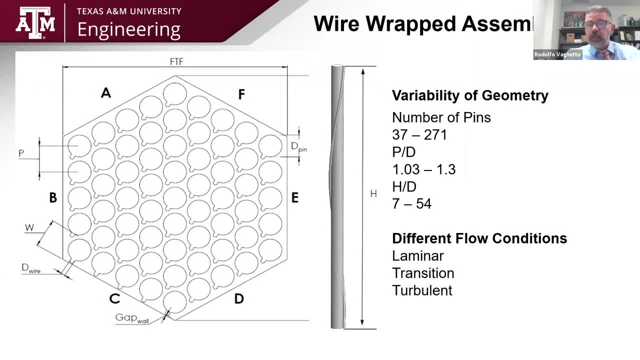 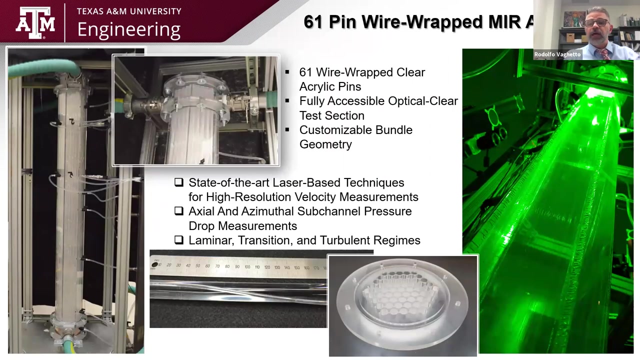 to validate the predicting capability of the existing correlation, For example the one for heat transfer or pressure drop, or I'm sorry but I need to- But also because they are important to the validation of computational tools like system-level code, sub-channel code and computational tools. 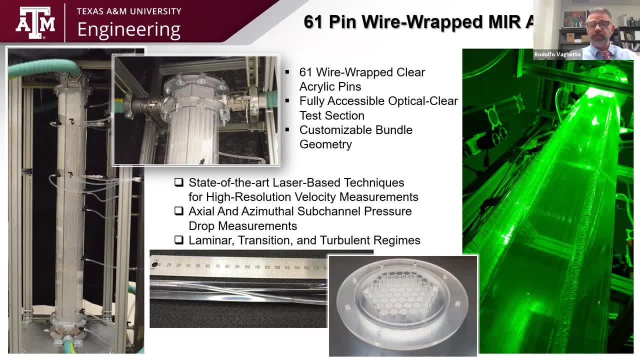 This is an overview of our test section. So the facility and the test section was designed and constructed under a project that- a collaborative project with TerraPower, Arriva from Atom and Argonne National Laboratory. So we. The test section is a 61-pin wire wrap replica. 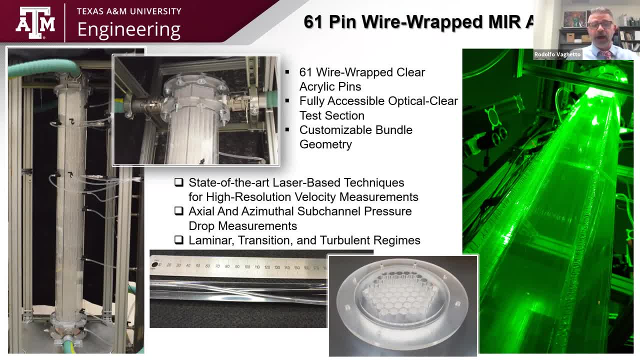 It is made of acrylic, It's a fully transparent, And the reason why we decided to make to fabricate this test section in acrylic is because we have employed an eye-fidelity flow visualization and measurements that I will discuss toward the end of this presentation. 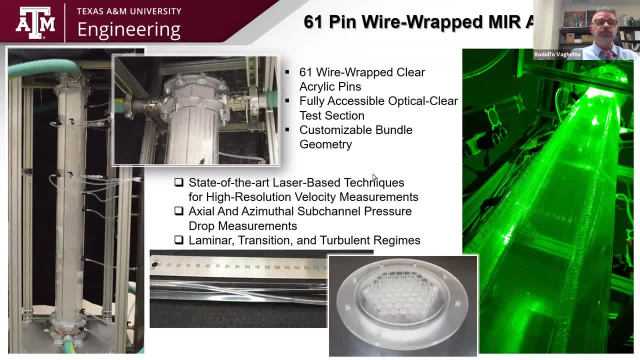 The test section is also equipped with pressure measurements. As you can see on the left, there are a series of pressure taps that are installed at different axial locations and different azimuthal locations to characterize the pressure behavior for the bundle. The test section is connected to a forced convection loop. 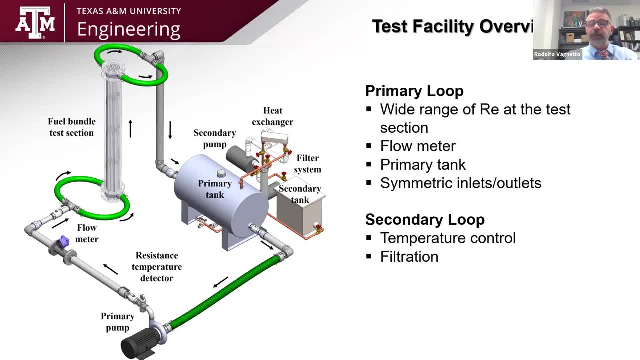 Here we have installed a primary coolant pump. The pump is basically used to establish the desired flow condition at the test section. And the pump is basically used to establish the desired flow condition at the test section Just to make sure the type of tests that we can conduct. 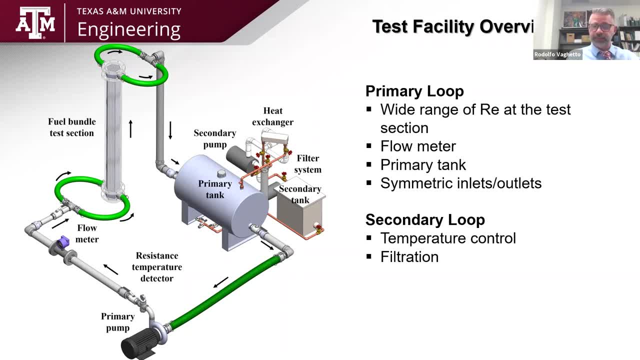 with our test section are what we call the isothermal tests, So we can conduct a test to study the hydraulic behavior, so the flow behavior within the bundle. We do not consider the heat transfer mechanisms, but still these experiments are important for the reasons I mentioned earlier. 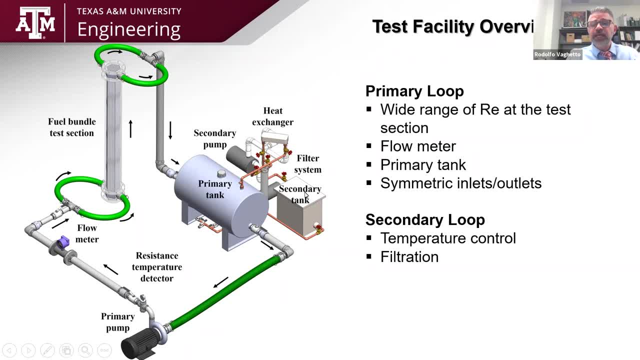 There is still a heat transfer system that is used to conduct the test. So the heat transfer system here, as you can see, there is a secondary system that you use to maintain the temperature of the primary loop under control. This is important because the fluid we use has specific optical properties. 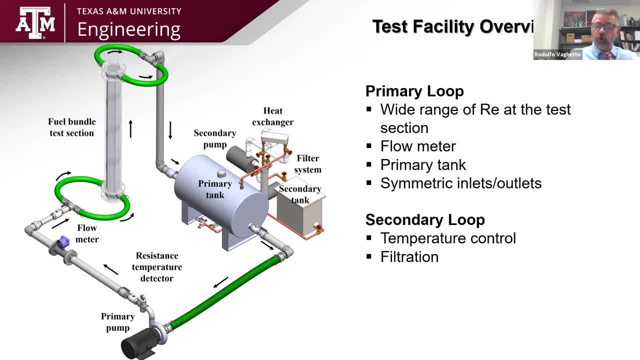 that change with the temperature. So it is important for maintaining the property of the fluid in altered to maintain the temperature constant. So it is important for maintaining the property of the fluid in altered during the tests. And this secondary system is also used for filtration. 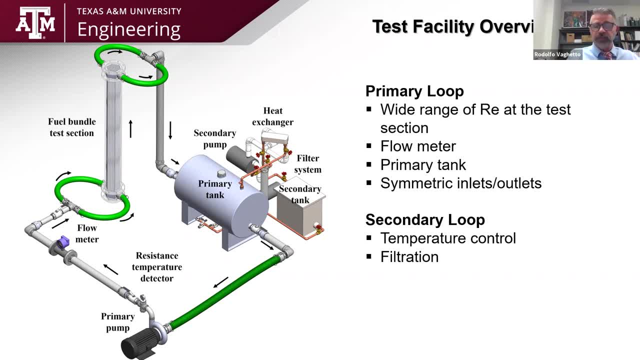 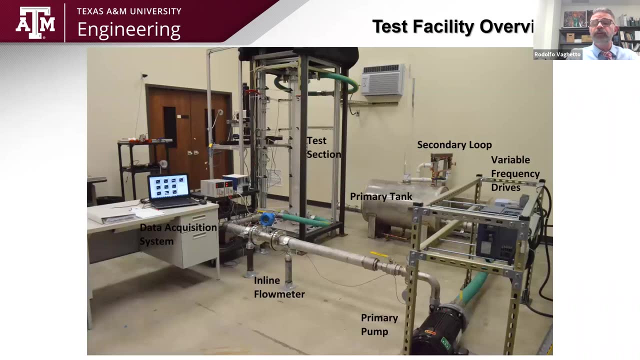 We have a system level measurement of the flow rate And, as I will show you later on in the presentation, we have also camera and the laser that are installed to conduct the flow visualizations. This is an overview of the test facility, with all the components that I just mentioned. 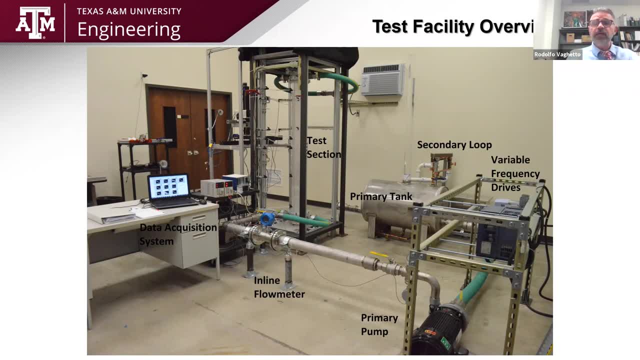 So I will not talk too much about it. I will talk more about the test facility. If you guys have any questions, you can ask me at the end if you are curious to know more about the test loop and the design of the test section. 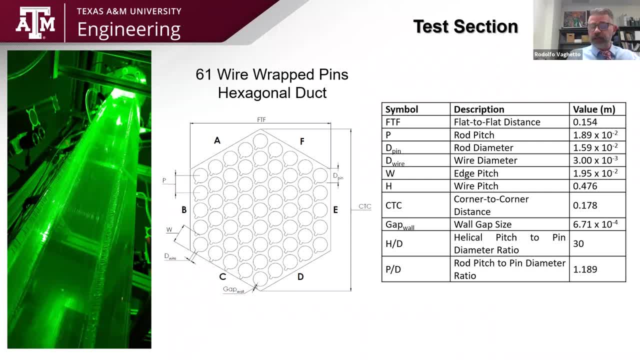 These are the geometrical feature of the bundle- are basically have been provided by TerraPower, So TerraPower provided the test specification. We went through a series of iterations because, since the bundle was built in acrylic, we had to face a certain engineering consideration. 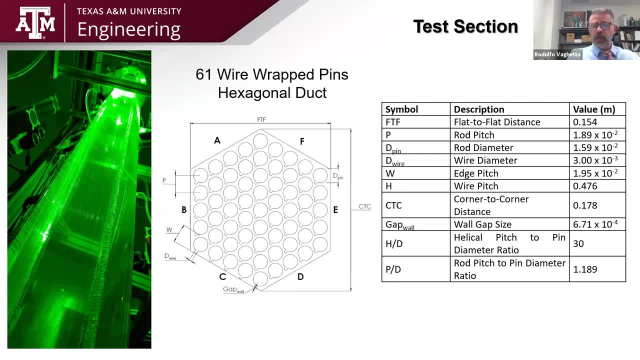 But these are the final dimensions of our test section. Of particular importance is what I mentioned before, the edge pitch. This edge pitch for this bundle is relatively larger compared to any other existing experimental test bundle of similar geometry, And it's because the vendor wanted to explore. 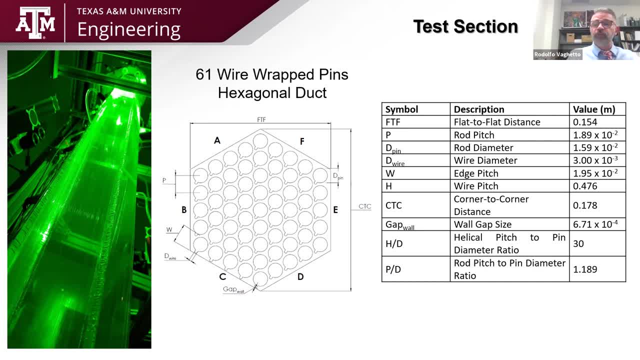 the ability to increase the edge pitch to further increase the lifetime of the bundle. During operation this bundle may undergo to thermal expansion and deformation of the pins and the duct. So having a larger edge pitch will allow to this thermal expansion, especially toward the center of the core. 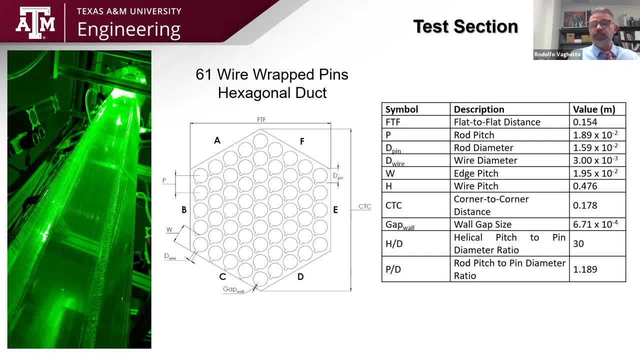 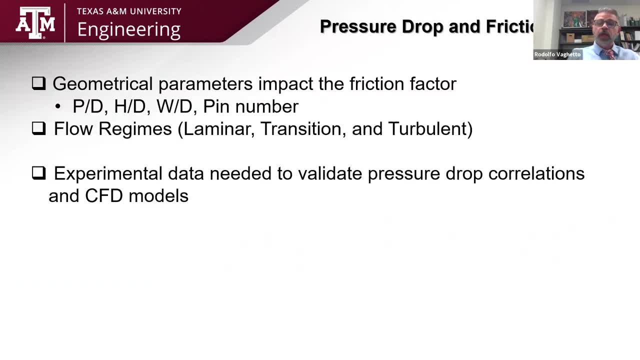 But again, you cannot work with edge pitch, otherwise you have to face a large amount of flow diverted toward the periphery of the bank. So, as I mentioned before, the combination of all these parameters and the variability of the parameters, like p over d, h over d, w over d, the pin number, the flow regimes, 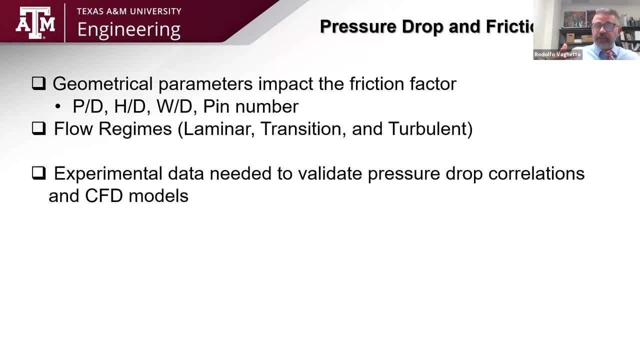 these are the main reasons why we have found this motivation to perform additional experimental tests, And there are different correlations available, for example, to predict the pressure drop and the friction factor in these type of bundles. I think you are familiar with the Cheng and Todrea's correlation. This is one of the most used because one of the most. 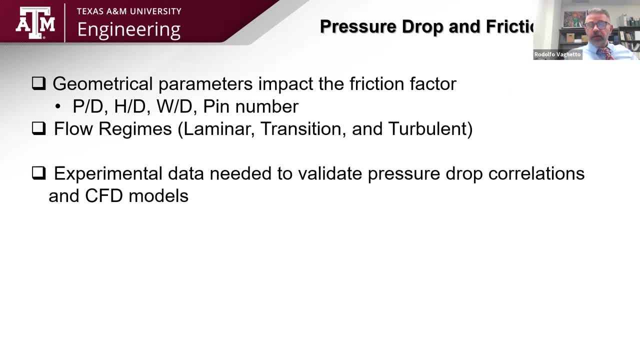 validated correlations available for designers to use, And these correlations are probably the ones that the larger amount of experimental data will go to for the validation or for improvement of the prediction. But recently also CFD computational tools have used this experimental data for validation of the 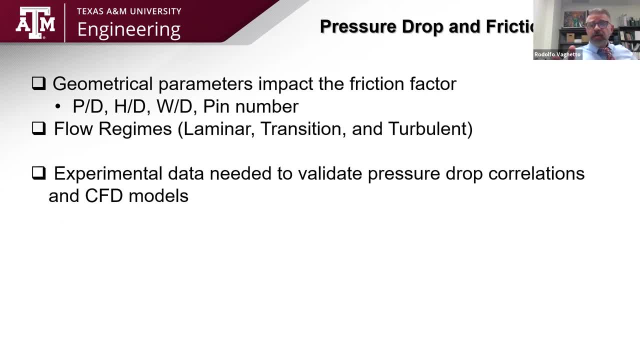 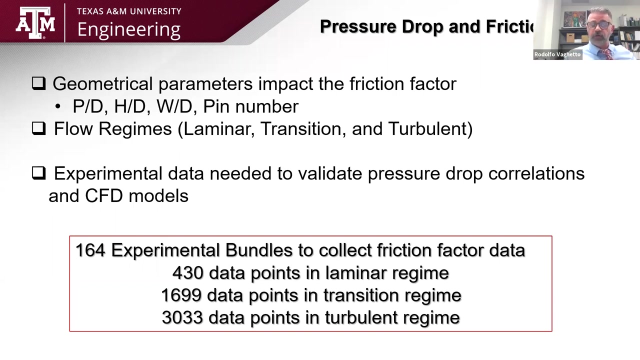 capability of these CFD models. Now the Cheng and Todrea's recently have done a very extensive literature review to identify the number of experimental test bundles currently available and the number of experimental data points that they could use to further improve their correlation predictions. And they have identified the 164 experimental test bundles. 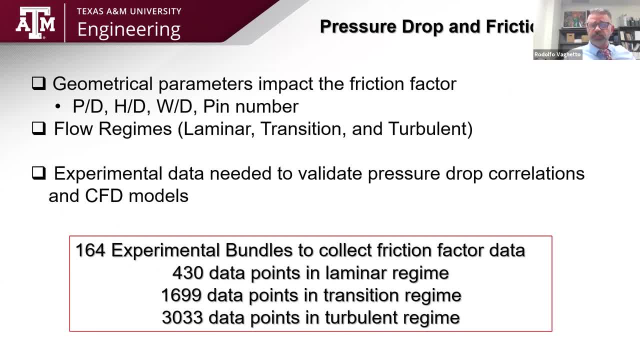 around the world, including the one at Texas A&M University, with hundreds of data points in the laminar transition and turbulence regime, But for the reason that you can see at the top of the slide, these data points may appear to be a lot, but in the reality we really need experimental. 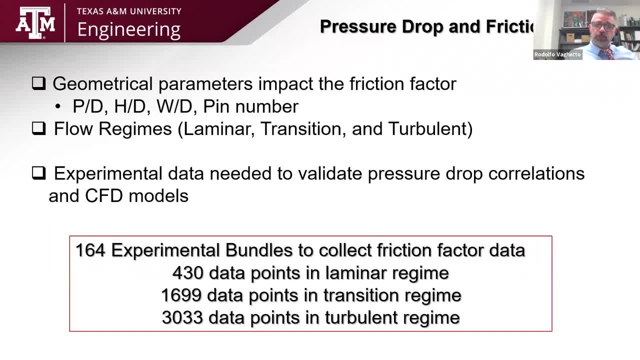 data. If you can see here, for example, the laminar regime has not been really explored because historically researchers have focused more on the turbulence- turbulence regime and then transition, But laminar regime of ease of interest, and developers of correlation like Cheng and Todrea's have found data points in the laminar regime. 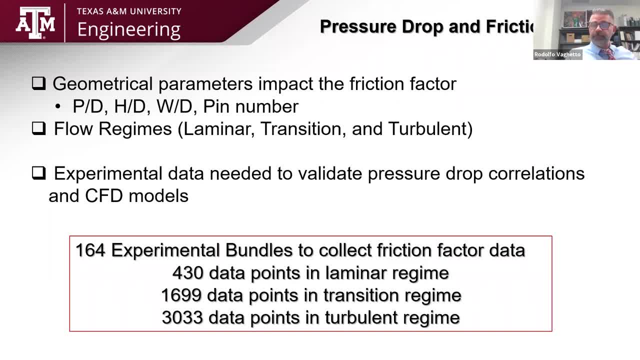 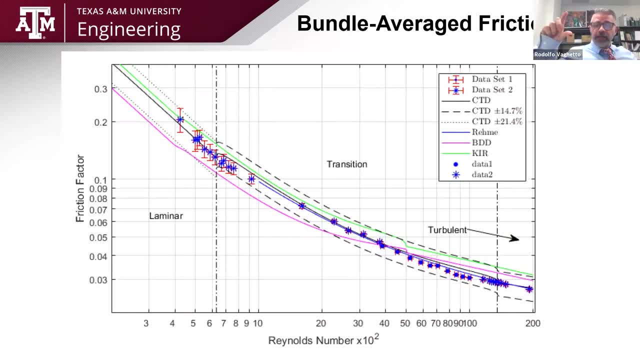 useful for improving the predicting capability of their correlation. So by reading the pressure drop over a one-wire pitch on the side of our test duct and we measure the pressure drop as a function of the flow rate, then we normalize the pressure drop with the bundle average kinetic energy and we plot in a log-log. 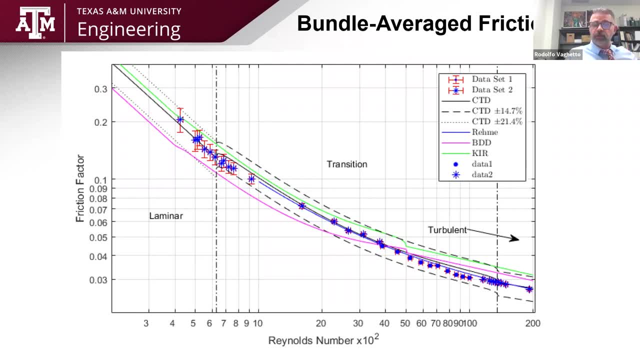 scale the bundle average friction factor with the bundle average Reynolds number and you see all the experimental data set that we produced a few years ago. compared with the prediction of selected correlations And, as you can see here, one of the things that we have noticed is that the Cheng and Todrea's correlation- it's a correlation proposed in the 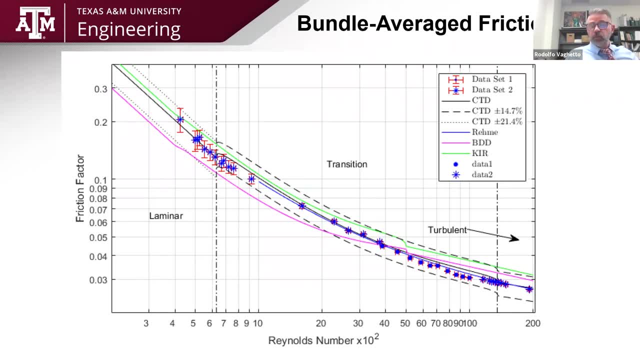 middle 80s have a good agreement with the trend of the experiments for our test bundle in, basically in a wide range of Reynolds number investigated. There are a few other information that you can get from this slide, but I'm going to stop there. So thank you very much, Thank you. 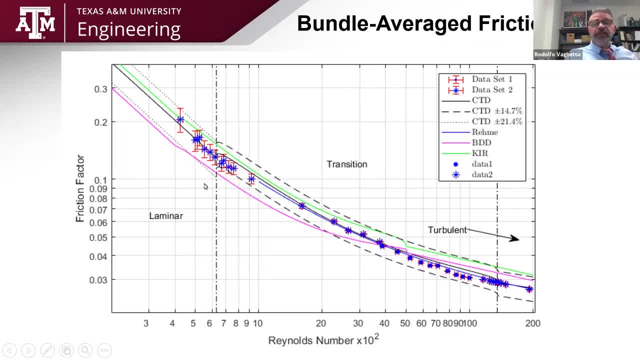 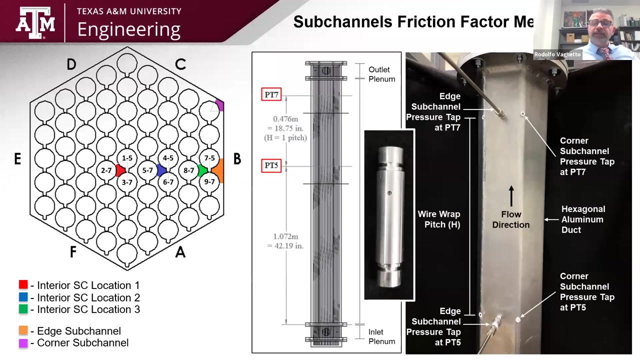 Thank you very much, Thank you very much, Thank you, Thank you very much, Thank you very much, Thank you very much. So this information is another information that is important for validating the correlation performance. One step forward in our experimental process was to go a little bit more in detail and instead. 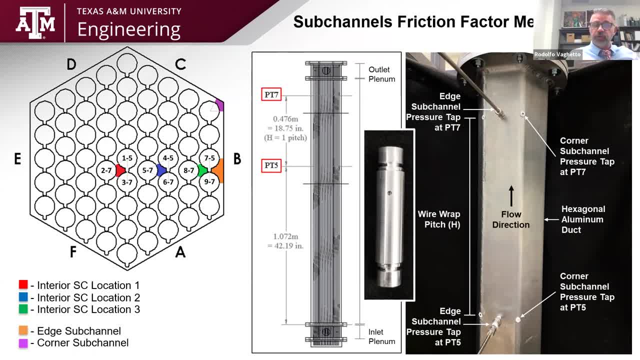 of analyzing the bundle average friction factor. we tried to be a little bit more creative and to fill the experimental data with the bundle average and the bundled average friction factor data needs, specifically in the interior subchannel regions, As you can see in the left side. 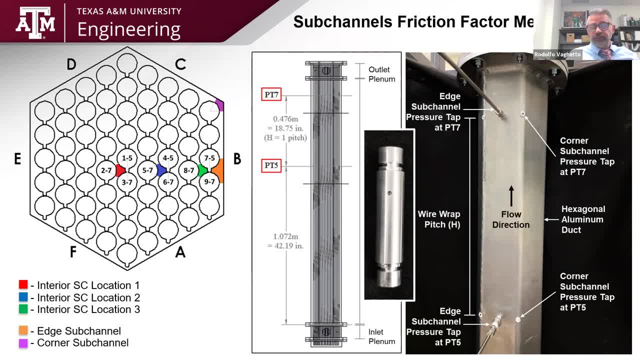 the subchannels are not all the same. As a matter of fact, Cheng and Todreas have identified the three types of subchannel: The interior subchannel, the one that here are identified with the red, blue and green colors. The edge subchannel, the one near the wall. 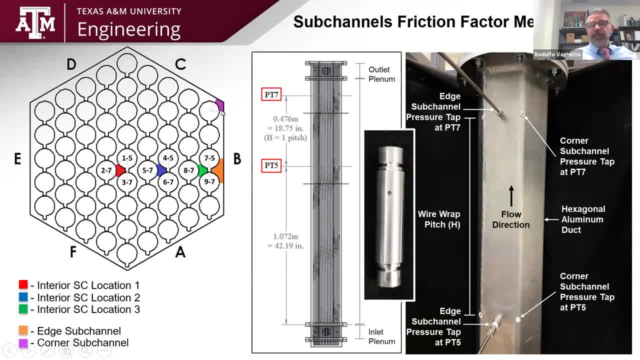 in orange and the corner subchannel And their prediction of the bundle average friction factor. it's a weighted sum of the local friction factor for interior edge and corner subchannel. So now, if you think about all the large number of experimental data that I mentioned earlier, 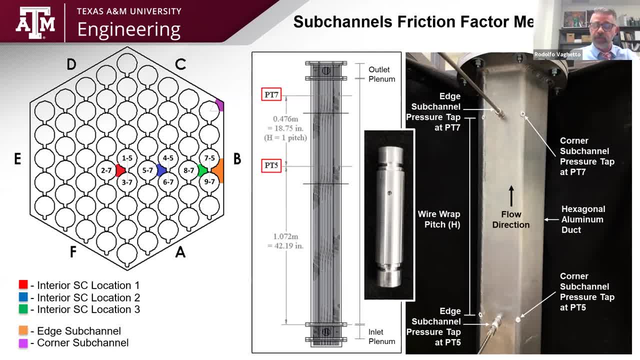 those are experimental data for bundle average friction factor. But if you count the number of experimental data for interior subchannel for local friction factor, then we want to say that the experimental data we have produced are really unique. So we have done some minor modification. 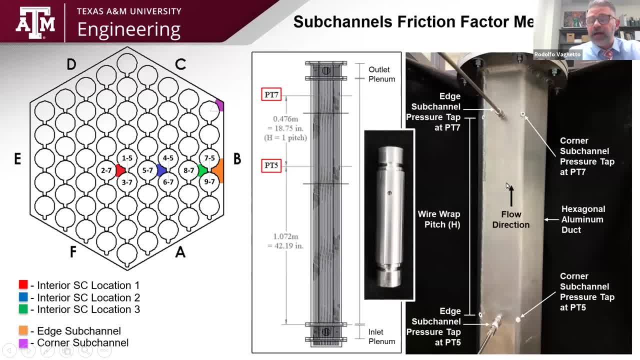 The first thing is we replaced the acrylic duct with an aluminum duct, and this has allowed us to create additional pressure taps at the corner and at the edge. Then we created, we designed and machined in our lab these rodlets that allowed us to measure the pressure. 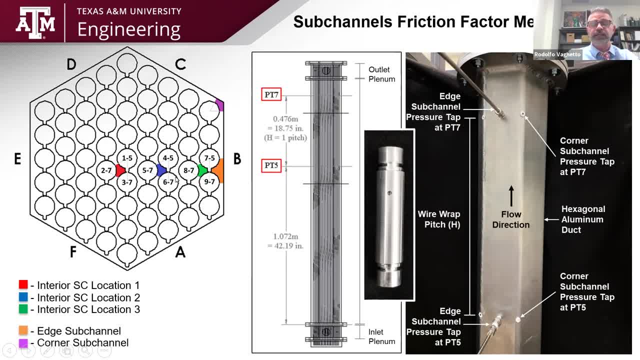 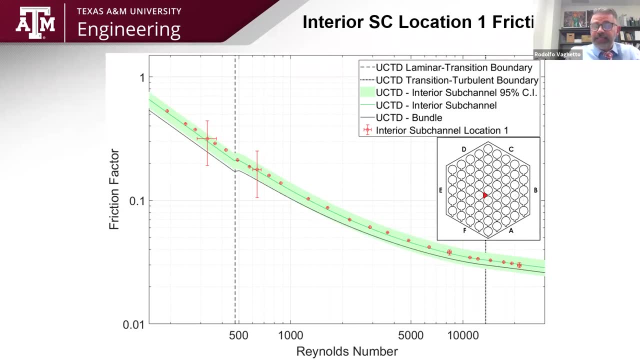 at different azimuthal locations, as you can see here in this map on the left. And so we measured the pressure drop, we normalize it again and we plotted as a function of the local Reynolds number And we were able to show the interior, the local friction factor. 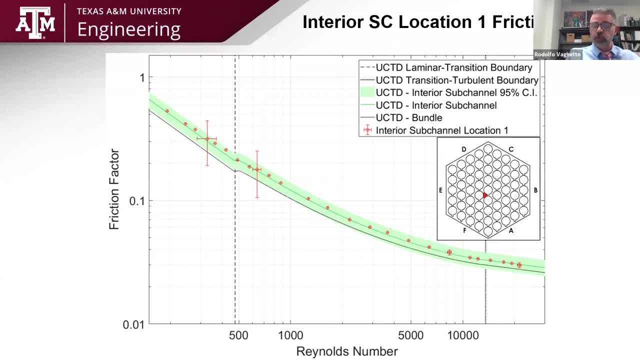 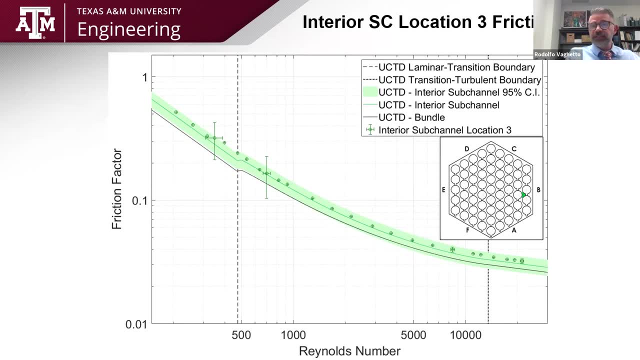 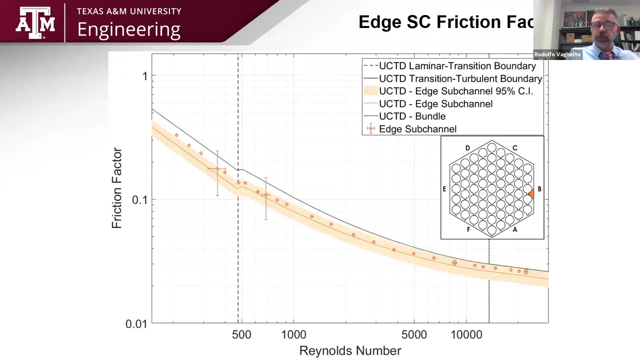 for three different subchannel: location one, location two and location three. And here what we have noticed is that there are no statistically significant differences between the friction factor among the interior subchannel when moving from the center toward the periphery. But then there is also the prediction. 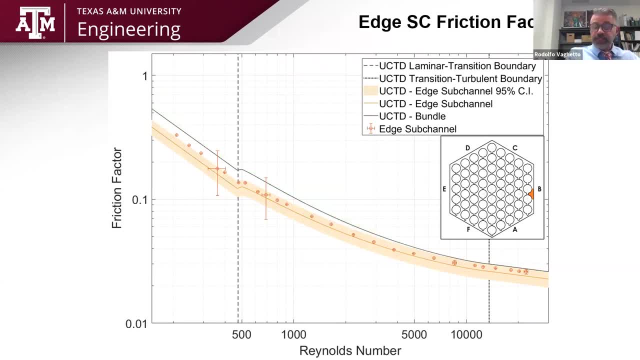 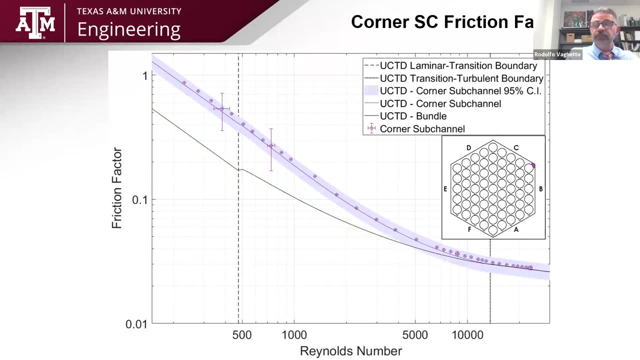 and the friction factor, the experimental results for the friction factor, friction factor for the exterior or edge subchannel and for the corner subchannel. In all the plots that I showed there are two continuous lines, one of the same color of the experimental data, for example, in this case for the corner friction factor, and these: 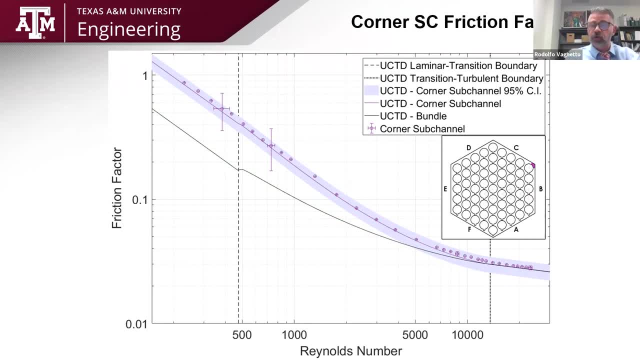 are the predictions of the corner friction factor of the Cheng and Todras correlation, specifically the UCTD, which is an updated version of the correlation that was proposed by Cheng and Todras in 2018.. And then there is the black line, that is the bundle average friction factor. that will 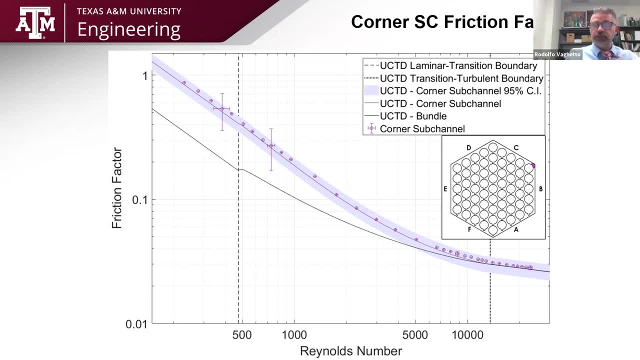 tell you what is the weight for each subchannel toward the bundle average friction factor. So this, basically, is one one of the most important points that I want to talk about today. So this, basically, is one of the most important points that I want to talk about today. 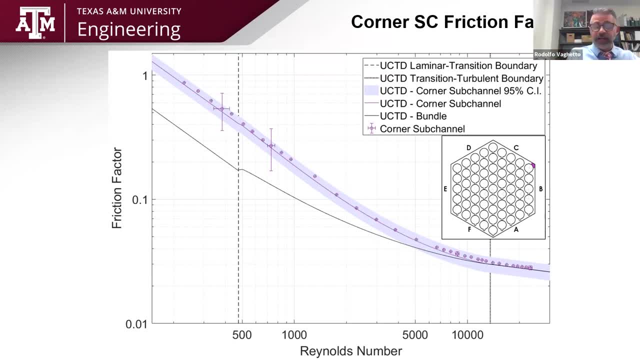 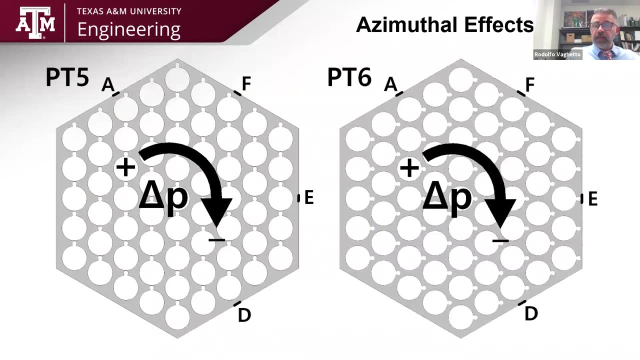 Of the most complex experimental activity we have conducted, only analyzing the bundle friction factor. We moved forward and now- I think I mentioned earlier- we were able to install the different pressure taps at different azimuthal locations. So with the bundle of this geometry, with the wire rotating as you move upstream and 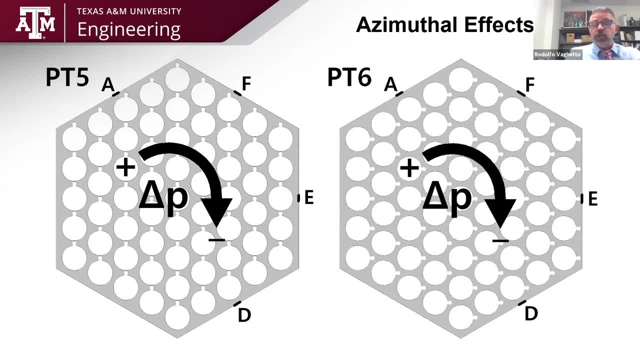 as you move with the flow, you will certainly realize that the distribution of the pressure across one specific cross-section may be of interest to analyze and understand, And the reason is because azimuthal pressure is important to know for estimation of the forces acting on the pins. 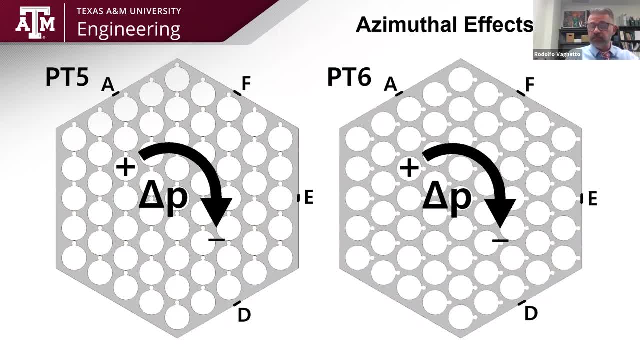 Subsequently, you can estimate the pin displacement or error, important of course for flow-induced vibrations. So what we did is we installed a series of pressure taps in the midpoint of four phases, The one identified with the letter A, F, E and D, at two axial locations. 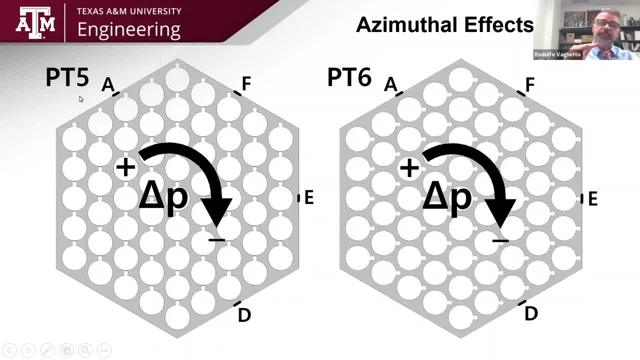 One. One is identified with PT5, it's in the full development region of the bundle and it's in a location where you have the wire that is pointing toward the corner of these two phases, A and F, And then we have another location, which is PT6, which is three-quarter pitch. 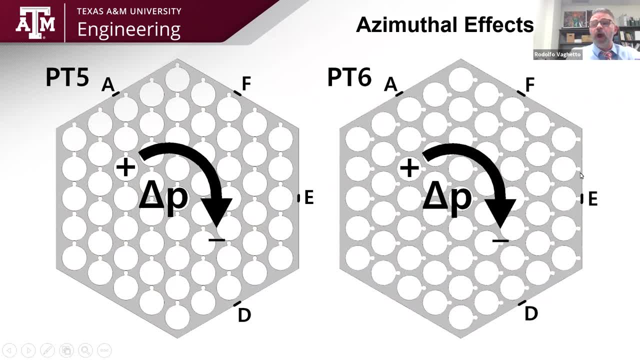 downstream PT5, and where you see the wire is facing orthogonal phase E. So we measured the pressure difference across each adjacent phase and then we found the different ways to plot the experimental results. And depending on how you plot the experimental results, we basically learn different information. 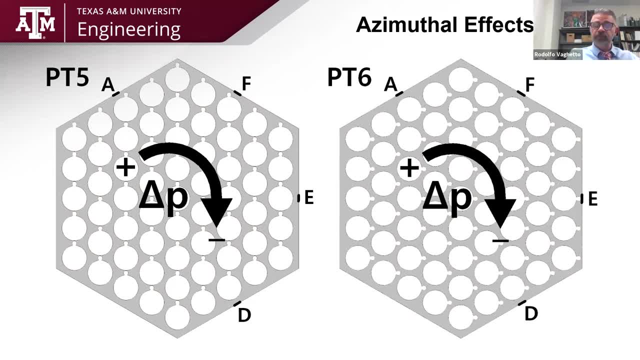 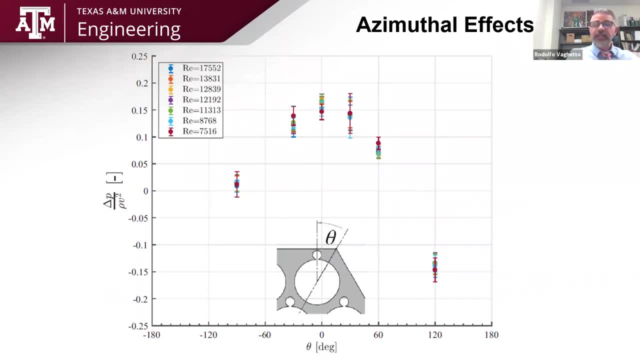 on the flow behavior in this type of fuel assemblies. One important takeover, for example, that we did by plotting the non-reactors, is to normalize the azimuthal pressure difference as a function of the angle of the wire compared to the corner between the two adjacent phases, is that there is a maximum pressure difference. 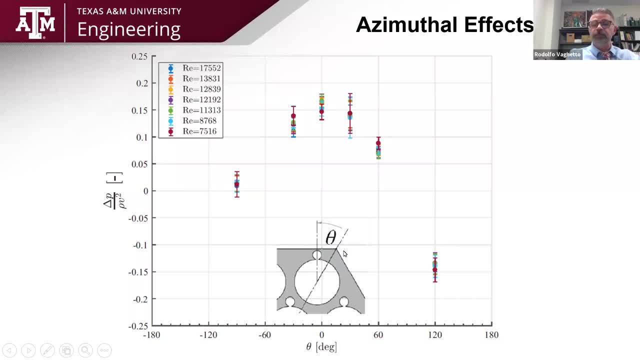 between the phases, when the wire is actually pointing at the corner, basically at theta equal to zero. We have also learned- and you cannot Maybe see in this plot by plotting in different configurations- is that when you increase the Reynolds number, you have a larger crossflow and the crossflow impacts the pressure distribution. 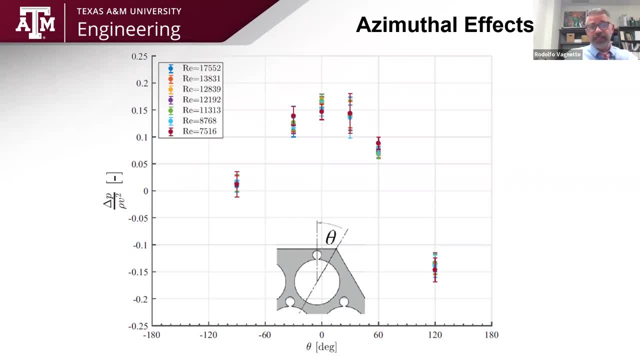 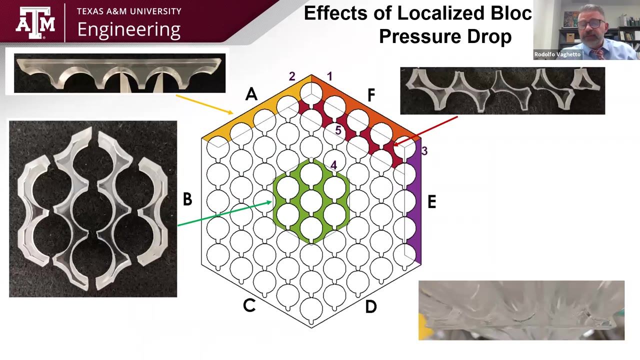 across the same plane. So the Reynolds number that is normal to affect the bundled axial friction factor in the reality will affect also the pressure distribution at each cross-section. One of the last activities that basically kept us busy for about two or three years now is 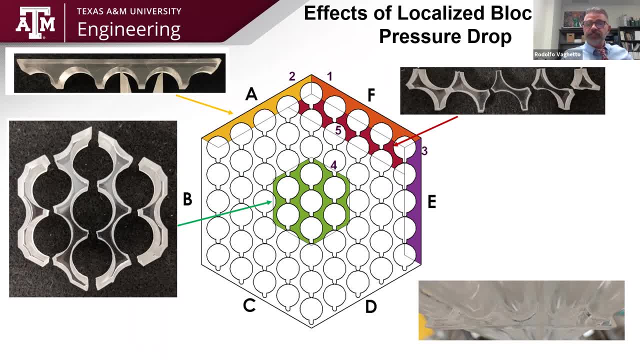 the estimation of the effect that localized blockages may have on the flow behavior. And here I'm talking about pressure drop again, Because the flow area of this subchannel is relatively smaller compared to a typical light-water reactor design, this bundle are more prone to accumulation of debris in the 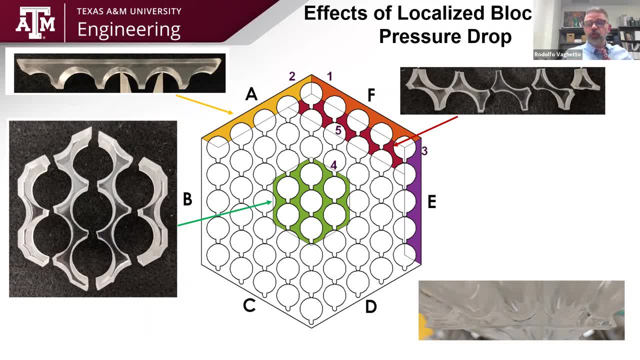 subchannel and, when the debris accumulate, may create a localized blockage. Now, with the reactor core instrumentation, there is really It's really very difficult to identify the presence of these localized blockages. But, as you can imagine, a localized blockage may have a very strong effect on the heat. 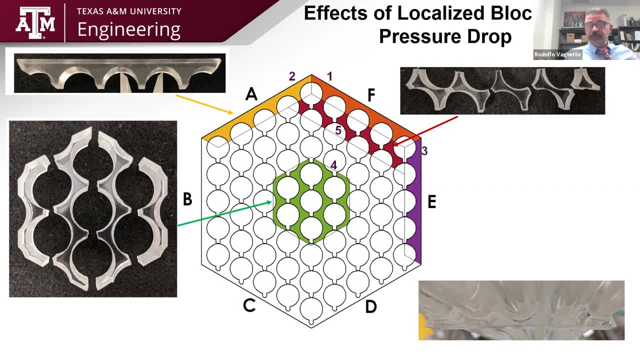 transfer and subsequently you can have a failure of a pin that basically can go undetected. So we used a systematic approach here, because you need to know that these blockages may not have a very regular shape and even the accumulation of debris may result in a blockage. 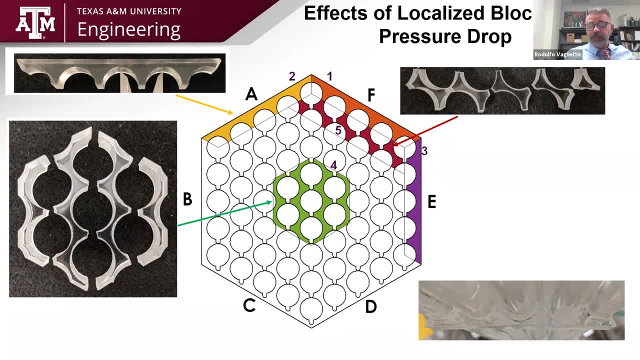 that is not a full blockage of the subchannel and it may have also a certain level of porosity. But if we wanted to study the effect of the blockage and specifically how the flow area block affected the pressure drop and how the location of the blockage may play a very 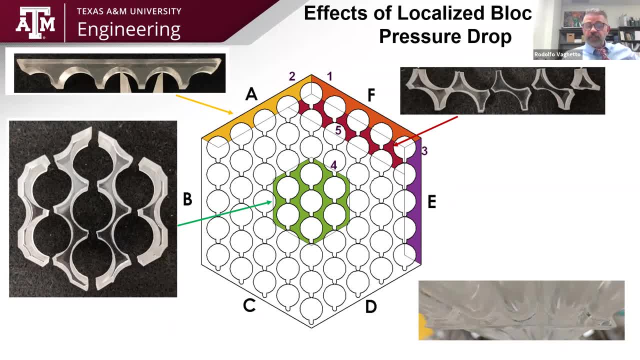 different role in the bundle friction factor. then what we did is we created very regular blockages that we were able to characterize with the conventional methods, like using caliber, but also with the digital methods. So we know the exact flow area we were going to block and we created different configurations. 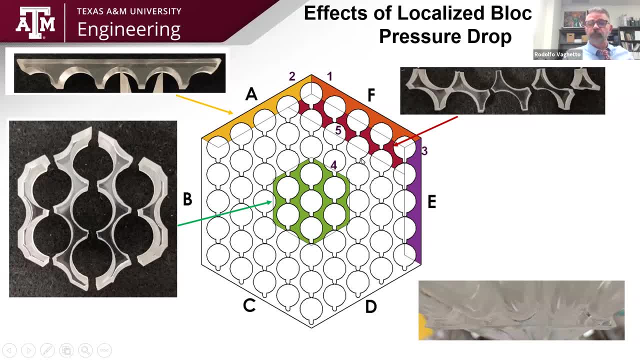 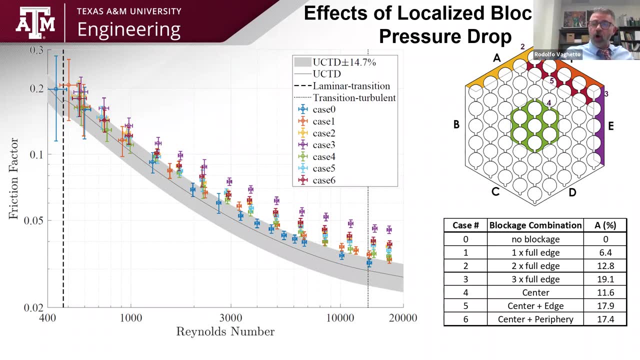 We have actually explored the six different configurations. The first one is a combination of blockages where the blockage has been located at different location in the bundle And by measuring again the pressure drop across one pitch within which this blockage is inserted. 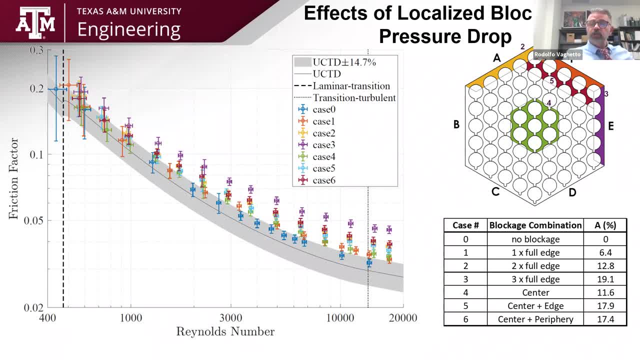 then we were able to study the effect that this blockage has on the bundle average friction factor. There are developers of correlations that are trying to draw the effect of the blockage and, of course, are interested in using this experimental data to include the terms in. 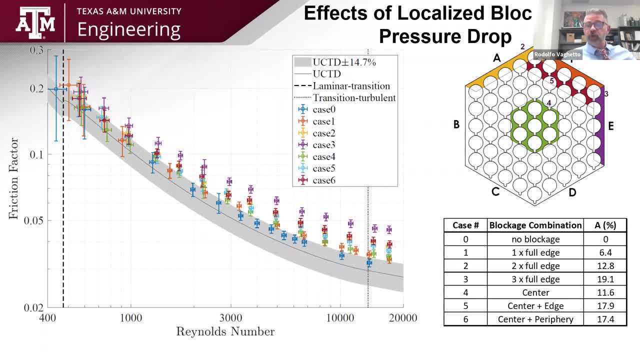 their correlation to account for the effect of blockages And, of course, these are experimental data that are unique and valuable if you consider the validation of a computational fluid, dynamic code. So here you can see all the cases analyzed, including what we call the case zero, which 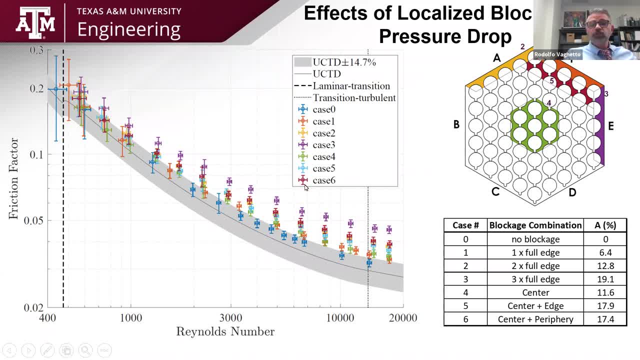 is the free Uh bundle without blockage, and they are all compared with the prediction of the change in progress which predicts that the friction factor with no blockage. So from here you can see the effect of these localized blockages on the bundle friction. 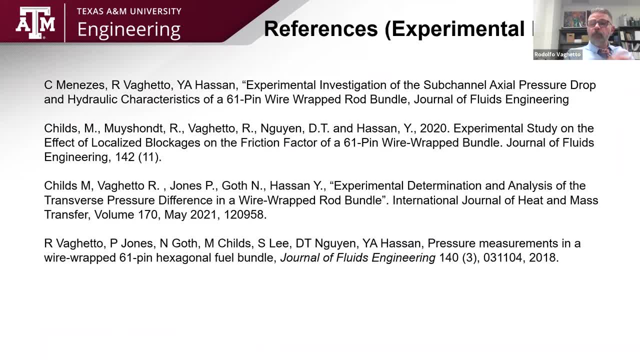 factor. So, if you want to know more about the experimental activity we have conducted, these are the list of articles that we have published. All of these are the list of articles that we have published. All of these are the list of articles that we have published. 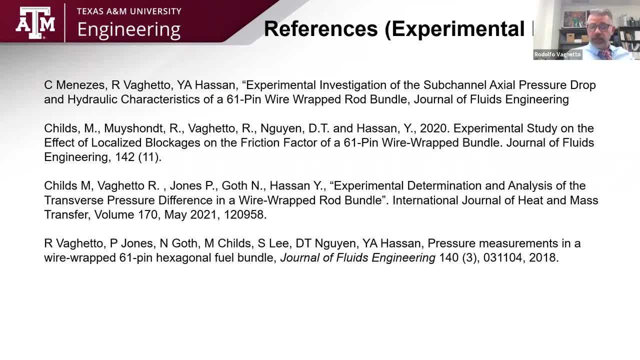 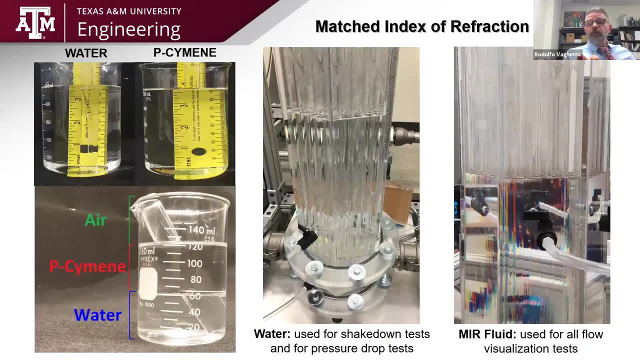 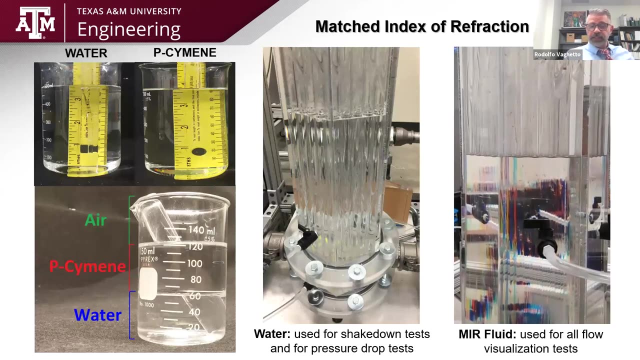 I have the only for the experimental pressure campaign. We have a paper that we have published for the eye fidelity velocity measurements that are going I'm going to discuss in the next two slides. So for some of you that are not, That are not familiar with the, the flow visualization techniques that we have adopted, the bundle. 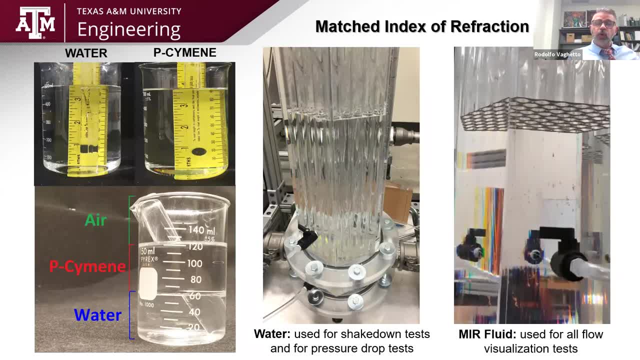 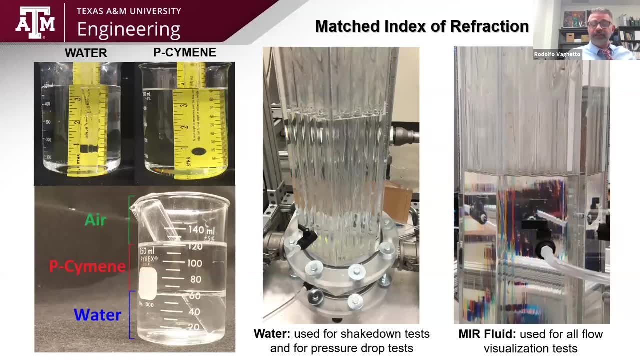 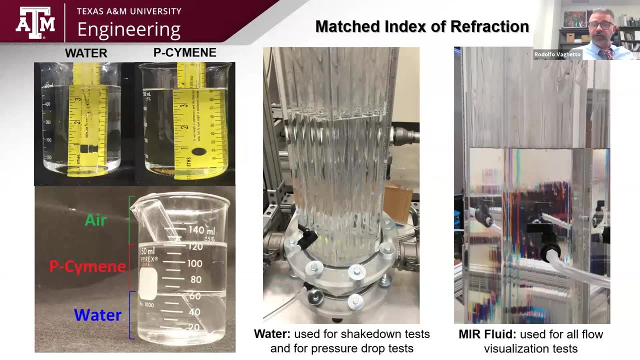 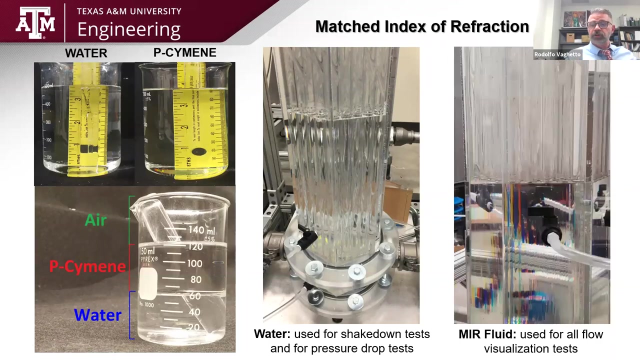 has been built In acrylic and we are applying what is called the matched index of refraction MIR technique. that consists of using a special fluid- it's called the pisamine- that has the same index of refraction of acrylic When you couple the liquid with a clear, solid material with the same index of. 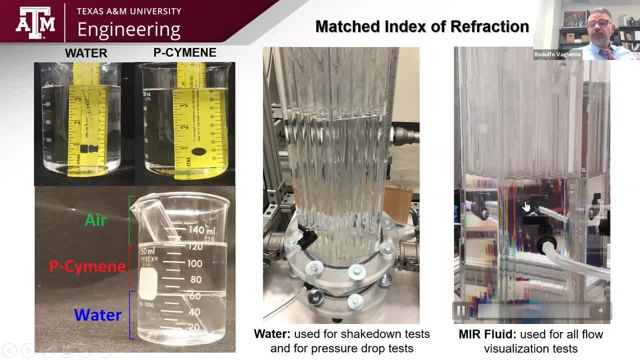 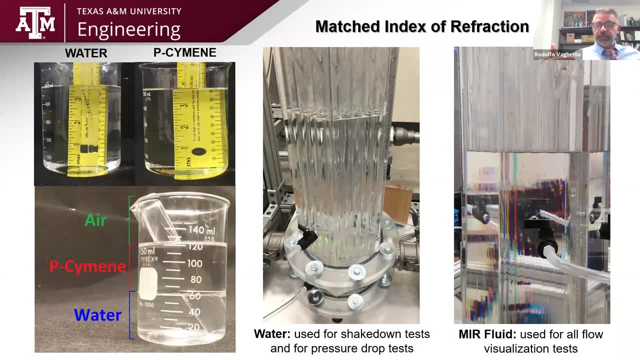 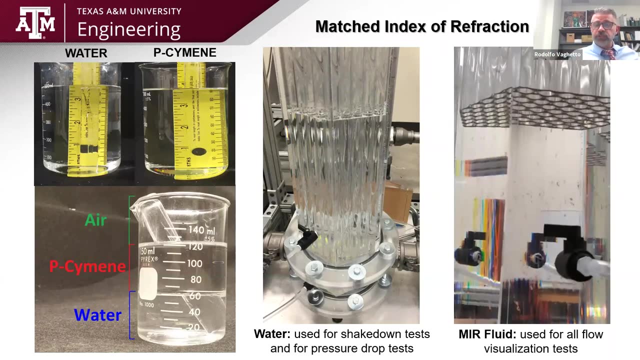 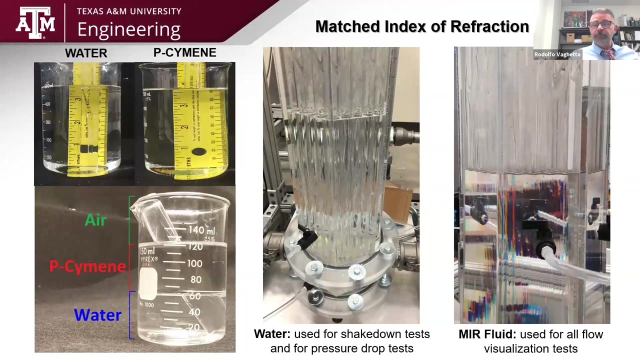 refraction. you have this clear feature of the bundle that allows you to visualize the flow not only near the wall of the duct but also within interior subchannels, And with some corrections and with some other algorithms that are in place in our lab, we are able to reconstruct the two-dimensional flow fields. 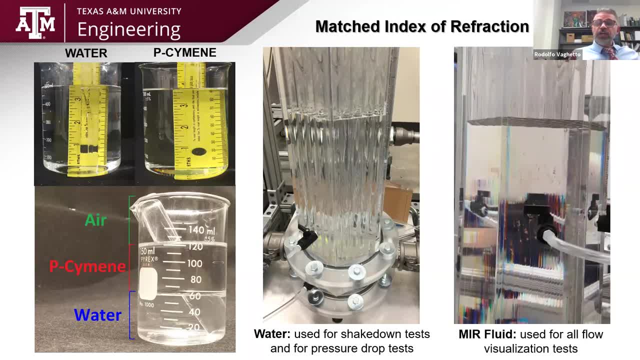 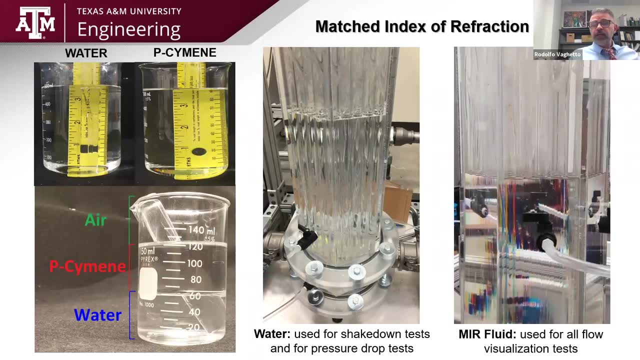 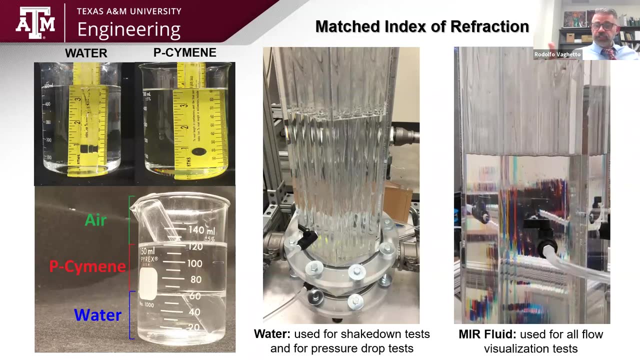 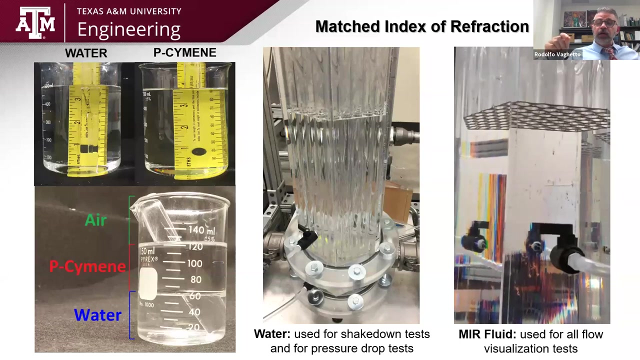 at different locations in the bundle. We combine this technique with what is called the particle image velocimetry. This technique consists on seeding the liquid with the small particles, having a laser sheet illuminating this particle and basically measuring the flow field by looking at the motion of the particles that are fatfully 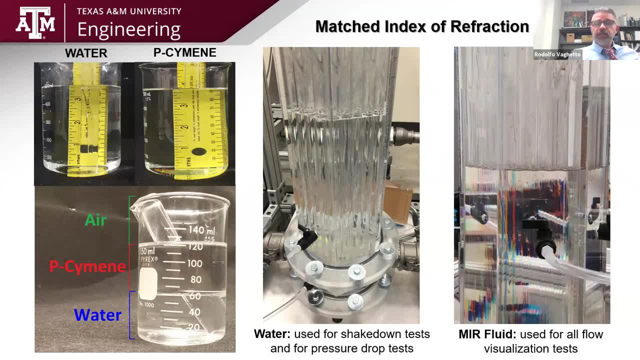 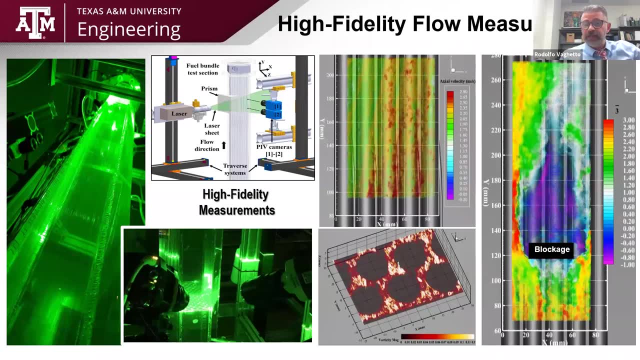 following the flow. in the bundle, And with these two techniques, we have basically produced a relatively large amount of experimental data of flow fields. These are more CFD-level experiments, In other words, these are experiments that can be used for validating the CFD. As a matter of fact, a selection of these experimental data are currently shared. 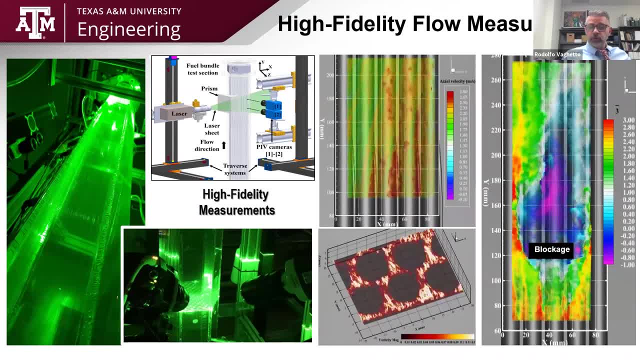 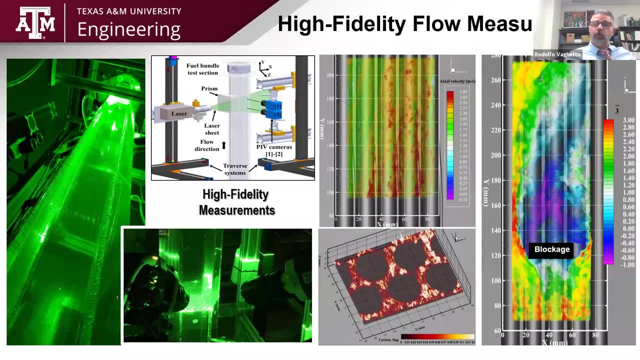 with the project I just mentioned, led by Dr Avramova. that will be part of an international benchmark exercise where people from around the world they use their own CFD methods and tools and see and use the experimental data to validate their computational capabilities. 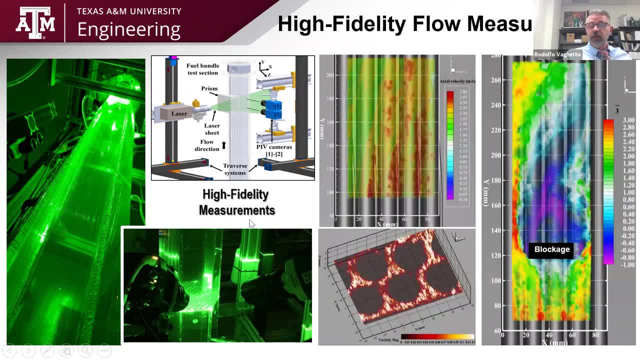 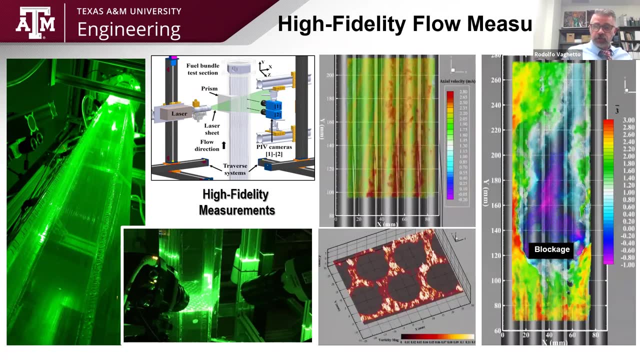 We have applied the PID for 2D PIV, 2D flow measurements. We have also applied what is called the stereoscopic PIV. that will give you the ability to measure the axial component of the velocity within a cross section on the bundle. And again, 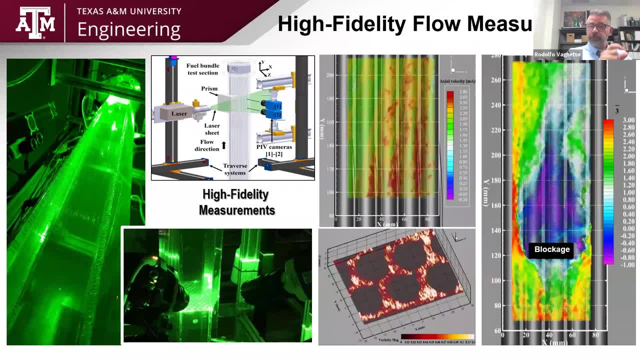 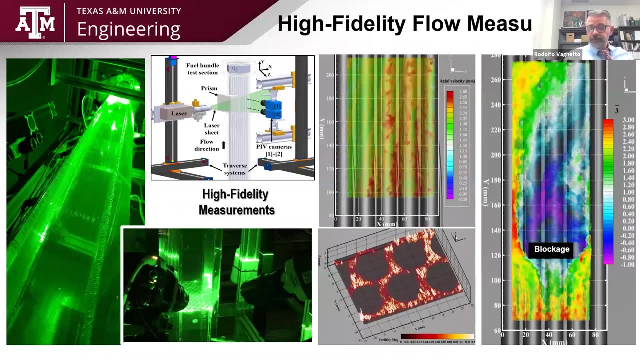 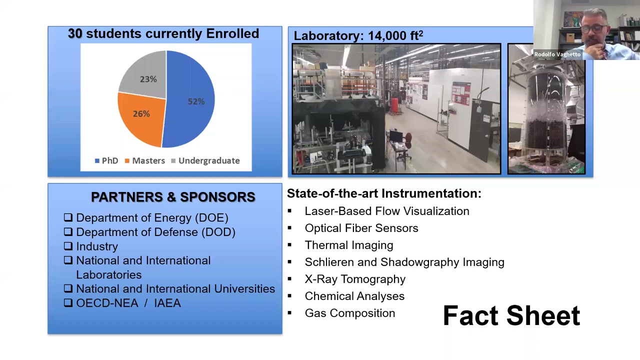 we have used the same technique adopted for measuring the pressure drop by installing localized blockages, but now showing how the flow structure is impacted upstream and downstream itself. This is the very last slide of the presentation. In the next few minutes, I want to spend just a few minutes to give you an overview of the capability of the Thermadralic Research. 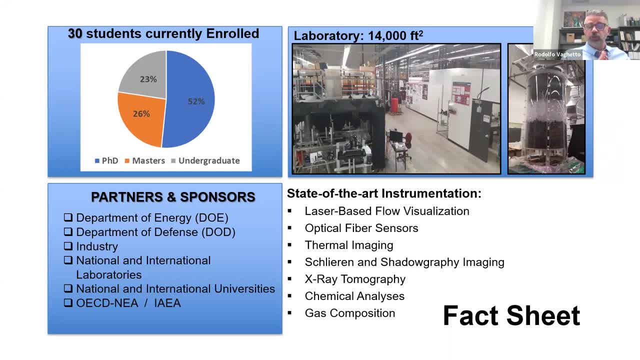 Laboratory, because we do a lot of research, and not only for this specific wire-wrapped fuel assembly. that, anyway, is one of the most active experimental and computational activities that we are conducting. So thank you very much, Thank you very much, Thank you very much, Thank you very. 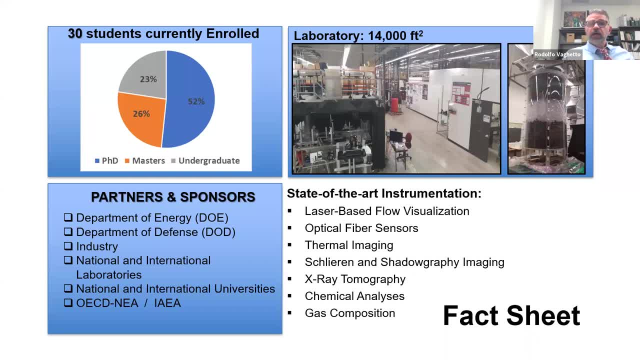 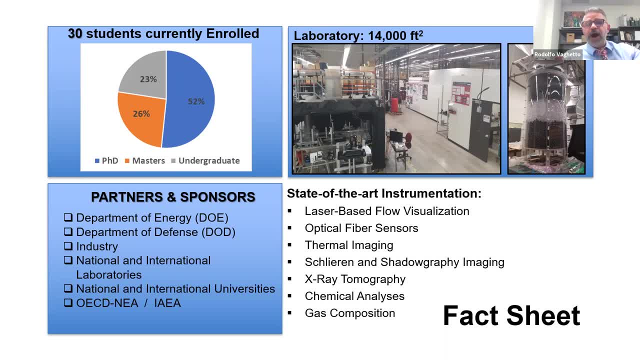 currently enrolled in our laboratory. We have partners and we work with the Department of Energy, Department of Defense. we have a strong collaboration with the industry. we we are fortunate to collaborate with national and international laboratories and university and and the some of the experimental. 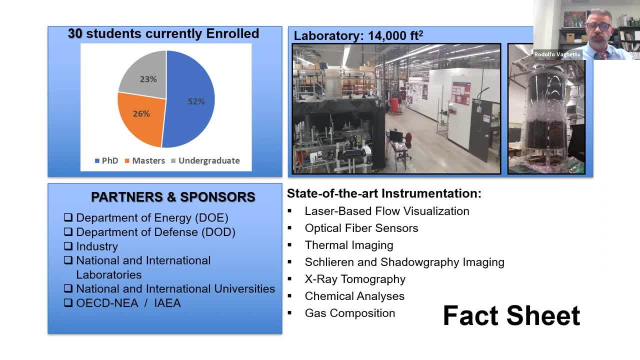 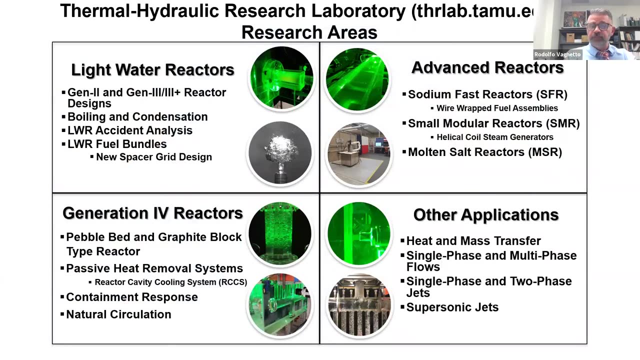 activity and experimental results we decided to share with the international benchmark, including the one that I just mentioned. right now, with Professor Abramova, We have developed techniques for measurement and simulations and we currently support the research and development in pretty much all the reactor technology that I mentioned in my slide number one. 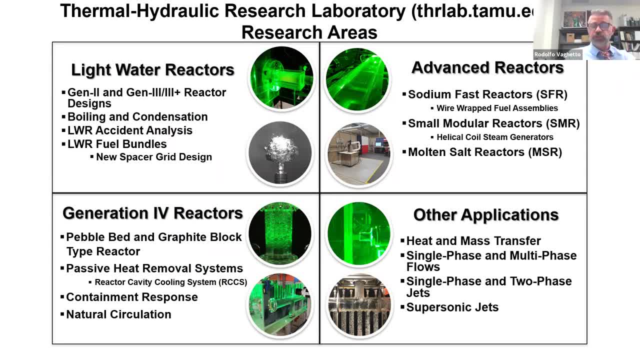 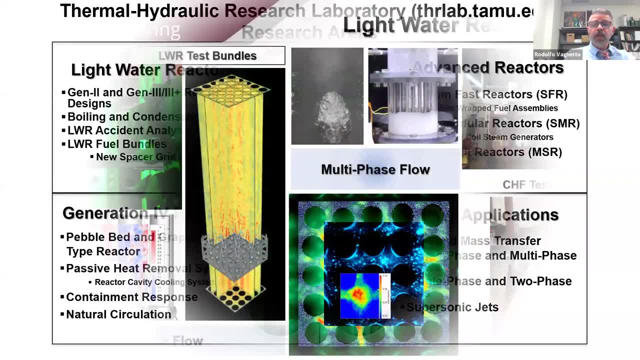 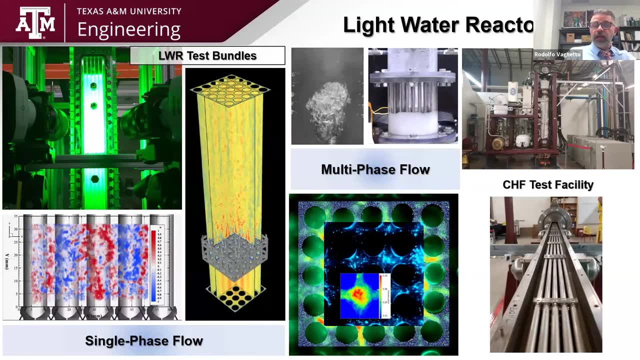 And we have in recent years expanded our research and development interest toward non-nuclear applications. We have supported the light water reactor industry. We have three light water reactor test bundles here in the lab: two that have been used for flow visualization and high fidelity measurements, and one 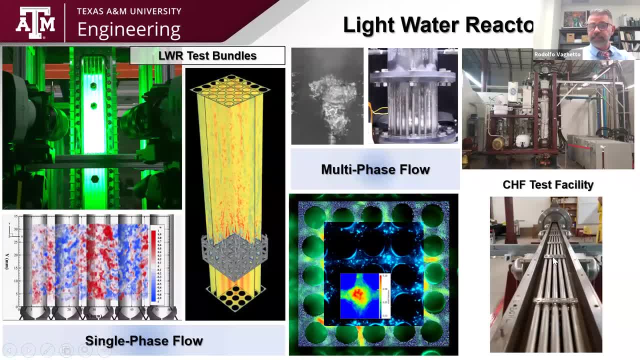 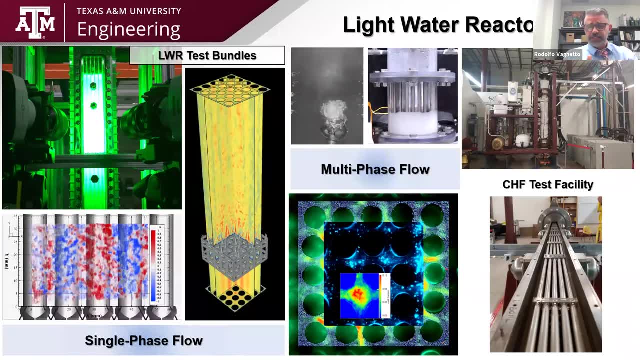 the one on the far right. that is a test facility that can operate at relatively high pressure and temperature for critical heat flux measurement. We have done single and two-phase flow measurement And of course we are engaged not only in the experimental part but also we do a lot of. 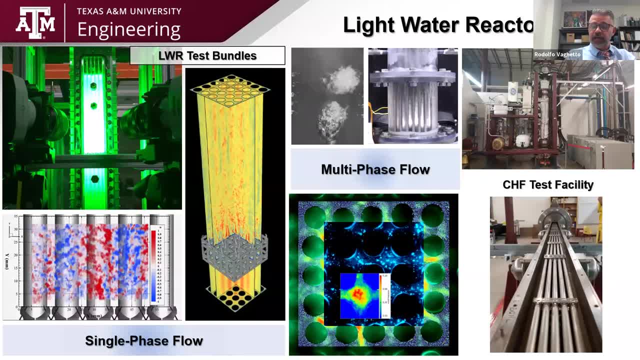 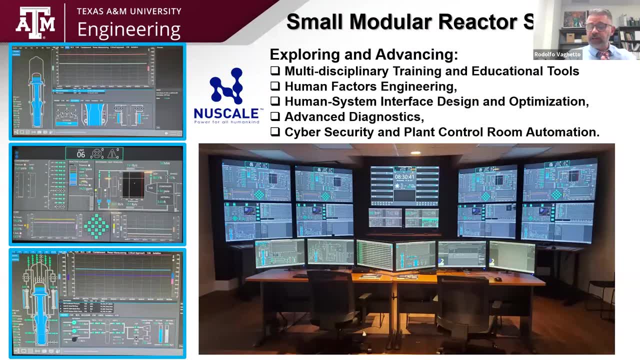 computational work with systems. We are constantly trying to develop how to achieve this, what we call an application level to a testing level. in CFD level codes We are hosting, we have installed a few weeks ago the new scale as small modular reactor simulator. 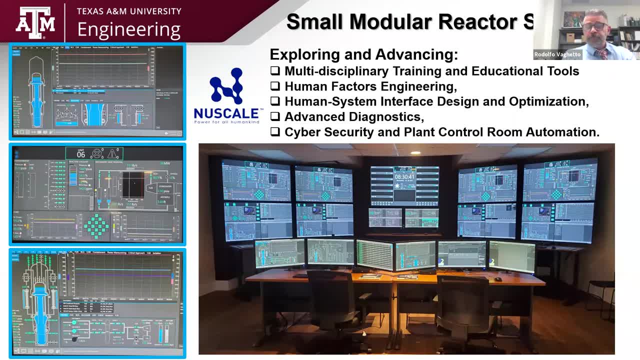 This is one of the simulator that the new scale have installed And it's actually an amazing tool, students to run. any accident scenario that are predefined accident scenario can be executed, but we have the ability to access basically every component of the power plant so we can basically 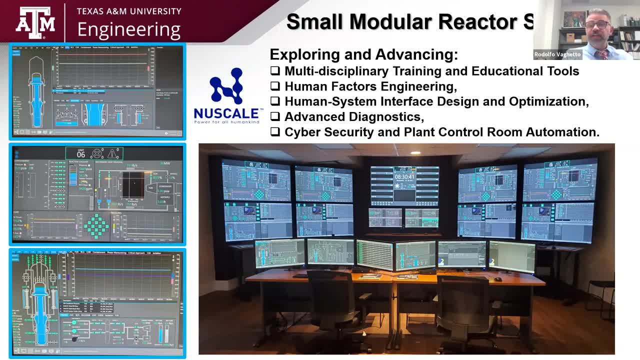 create any type of transient. We have access to the plant operating procedures so students are able to shut down the reactor, do refueling, start up the reactor from cold, shut down, change the power and do many other operations, and it's all digital. The simulator represents. 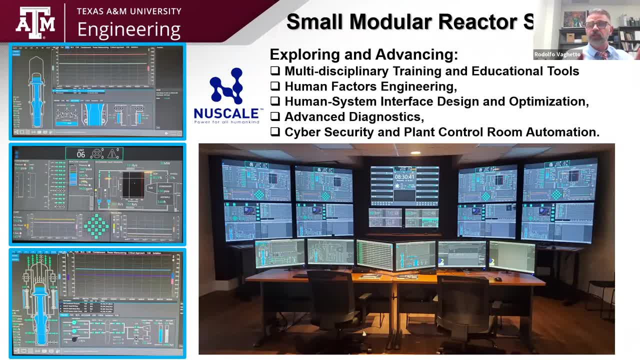 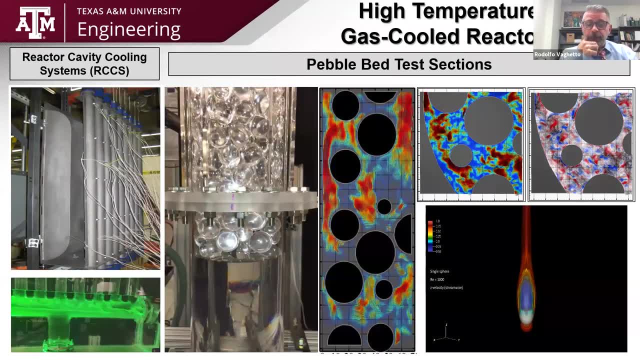 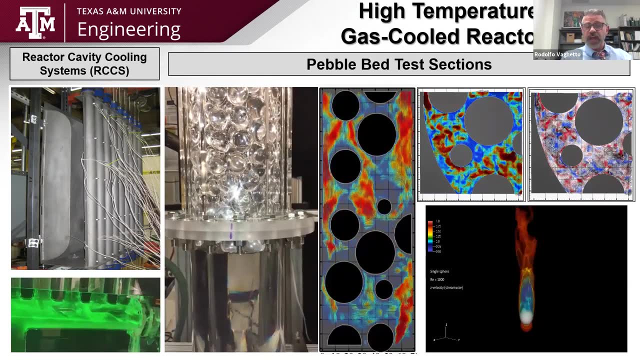 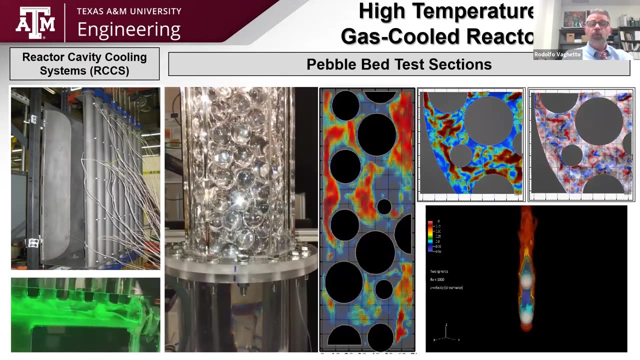 a power plant with 12 units and you can operate all the 12 units at the same time. We have also supported the development and research and development for high-temperature gas-cooled reactors. We have a test and simulation for pebble bed and graphite block gas-cooled reactors. We have also recently started an 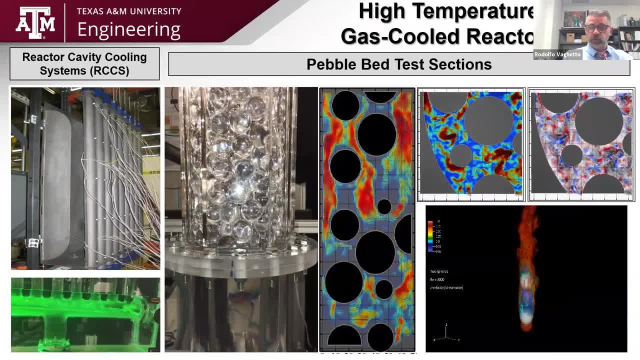 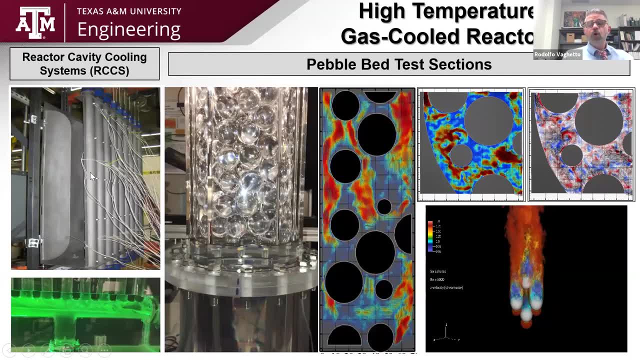 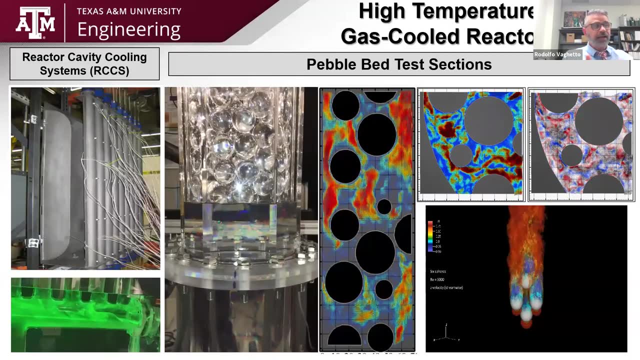 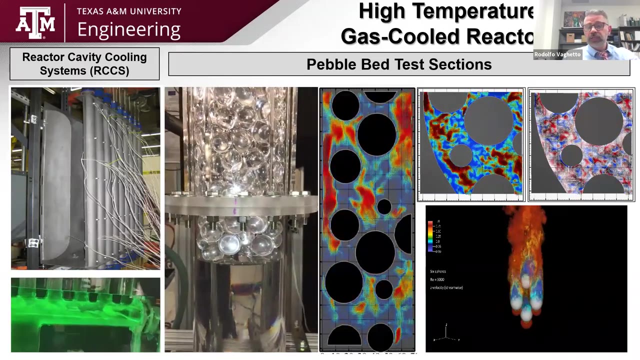 activity for a road bundle. gas-cooled reactors and the picture that you see in the movie on the left is one of the most used passive safety systems. that was designed for gas-cooled reactors, but there are now in more and more adopted for other reactor designs, including. 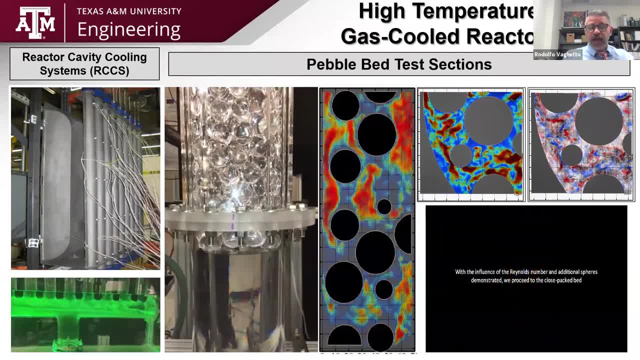 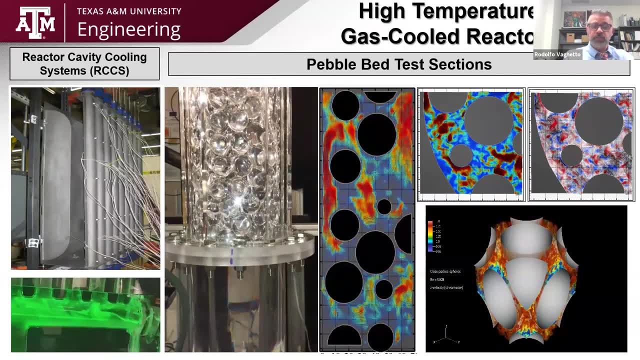 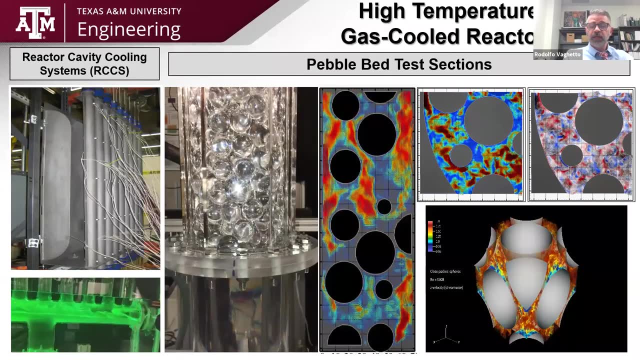 molten salt, for example. This is the reactor cavity cooling system and, if you guys know David Holler, Dr Holler was a student here and his PhD was basically conducted using this experimental facility, and we are currently working on molten salt reactors technology as well. 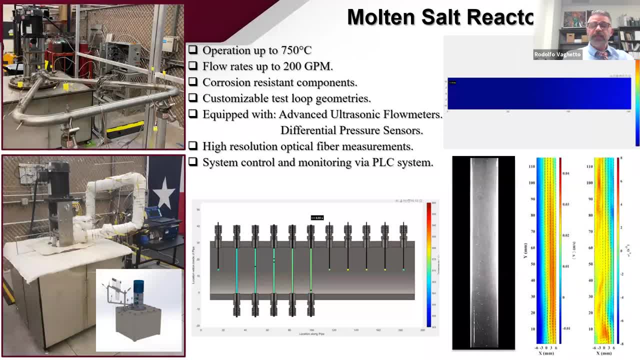 We have started this experimental activity approximately two years ago. We have built two forced convection test loop, as you can see on the left side. We have employed techniques for measured flow rates, pressure and temperature. We also conducted a flow snowballing physics to really understand that in high temperature. 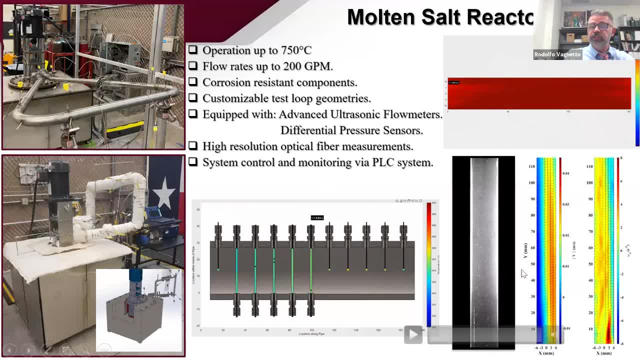 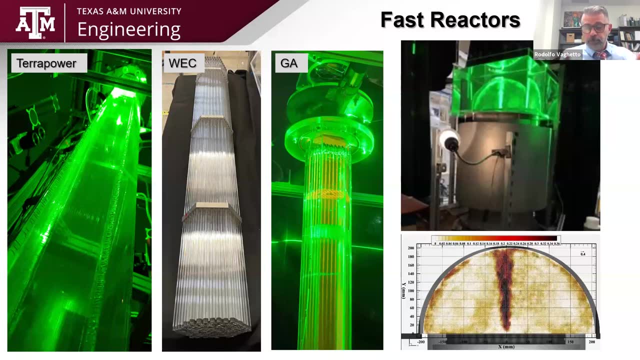 corrosive environment are very challenging And we have also conducted flow visualization using PIV in molten salt. Some of the molten salts, like Flinac, are transparent at high temperature And, as I mentioned, as I were and as I discussed mostly during the presentation, we are also 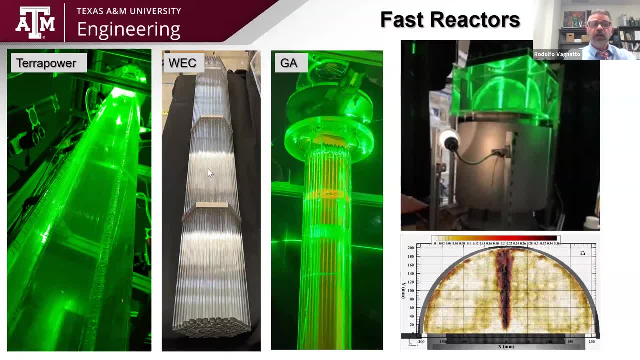 working on fast reactor technology, fast reactor bundles here, The one from TerraPower that I discussed during this presentation. we just built the bundle for Westinghouse Electric Company for their lead-cooled fast reactor design, and this is a 127-pin bundle. And then we have a bundle for the GA gas-cooled. 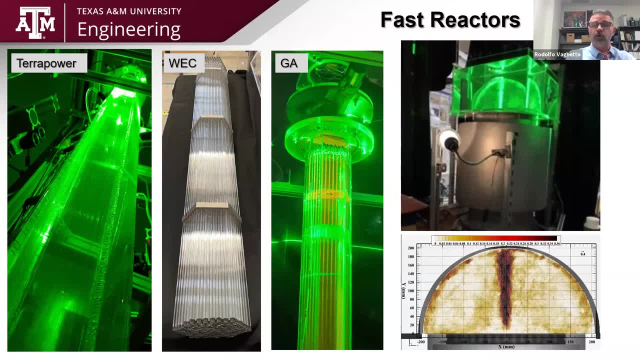 reactor. It's an 87-pin plus a central rod and this is already in operation. We have done some experiment and simulation also for the upper plenum mixing, which is one important phenomenon for fast reactors, And this is my last slide If you want to know more about. 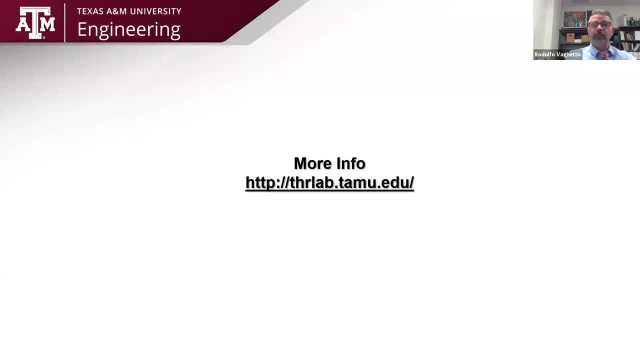 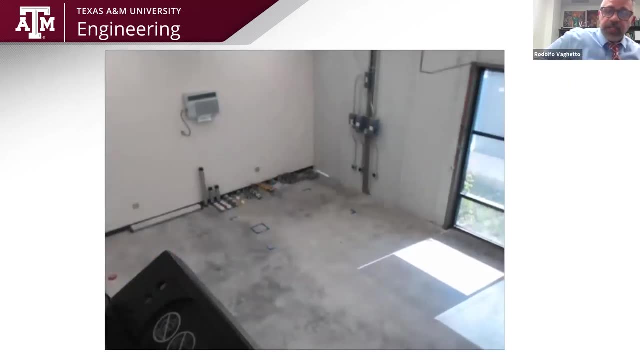 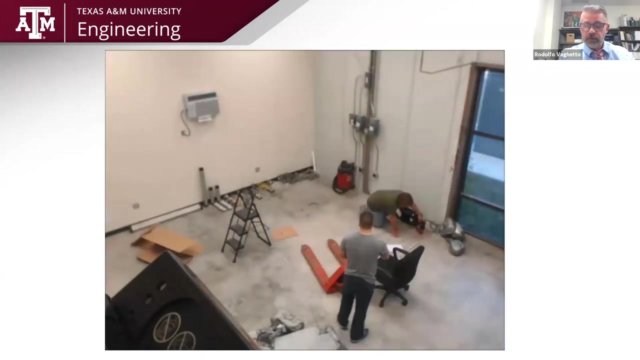 the activity, or if you want to know more about the wire-wrapped fuel assembly, you can go to the website of the Thermo-hydraulic Research Laboratory. and with this I will conclude my presentation And I will be – you will be very welcome to ask any question you have. 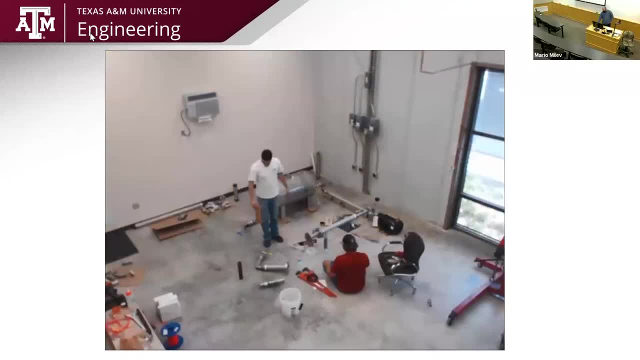 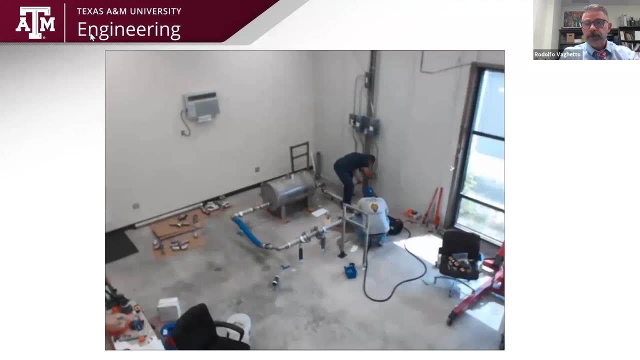 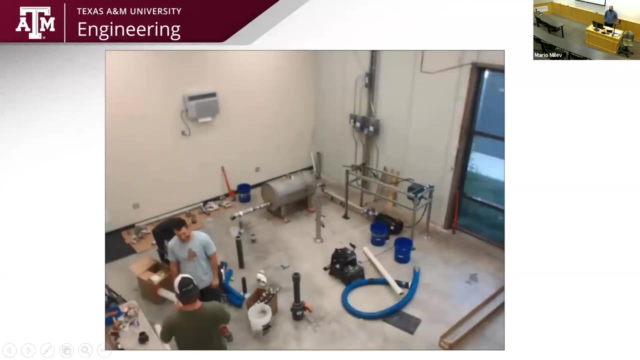 Thank you very much for your presentation. It was wonderful. Okay, so at this time I'd like to open the floor for any questions anyone may have. Either please raise your hand in the – and I can call on you from the participant list or, if you prefer, go ahead and raise. 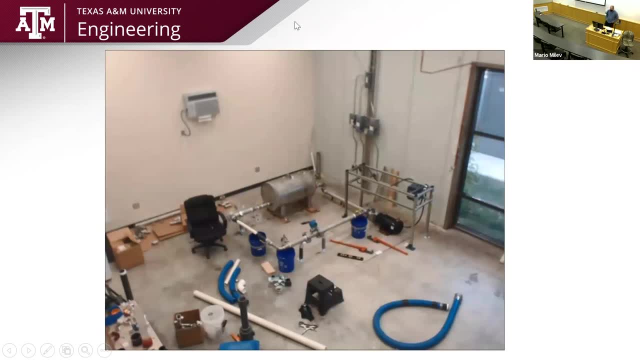 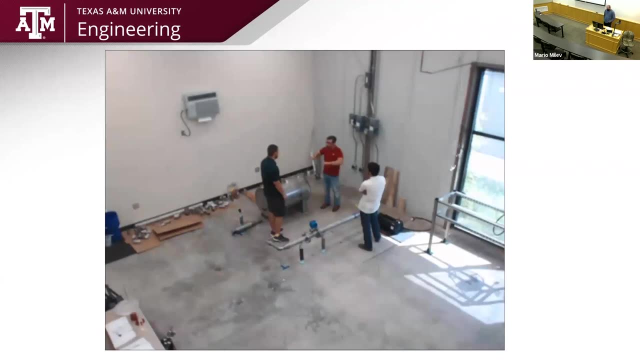 your hand, Thank you. I'll go ahead and post something in the chat and I can read it to our speaker. We're waiting for people – I was – I mean how much – so I'm not a reactor core guy, but I mean how. 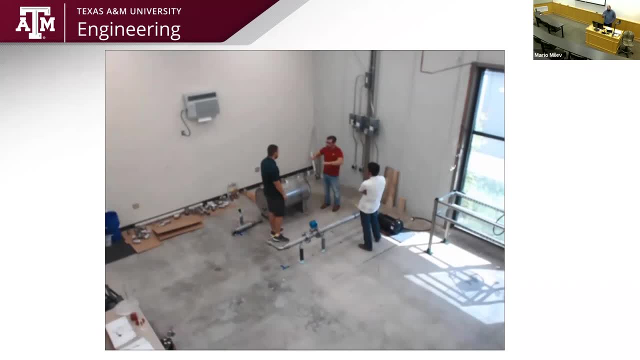 much torque do you get on those fuel assemblies Like I don't imagine those things are like a big propeller when you're spinning the – spinning fluid through there, especially something like a liquid metal. Is that an issue You need to – like the force that the flow itself apply to the bundle? 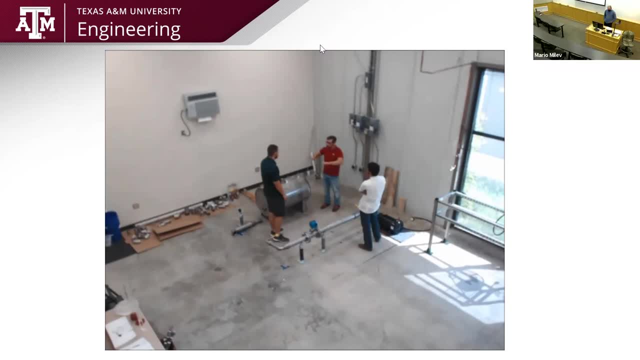 Yeah, When you move outward. Yeah, I mean, if they weren't bolted on the –, if they weren't bolted on the spacer, would they just spin? Oh well, so yeah, what you see here. of course, the spacers are usually meant just. 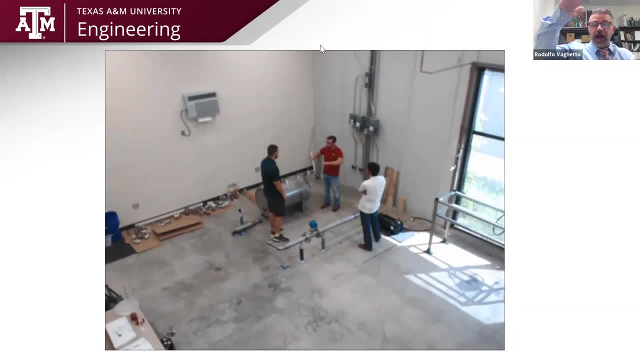 to provide space, but the axial – axial location of the bundle. it's meant by some upper and lower nozzles, So the bundle is itself connected to an upper and lower plane, So there is no way that it can move axial. So, yeah, you have a relatively large forces. 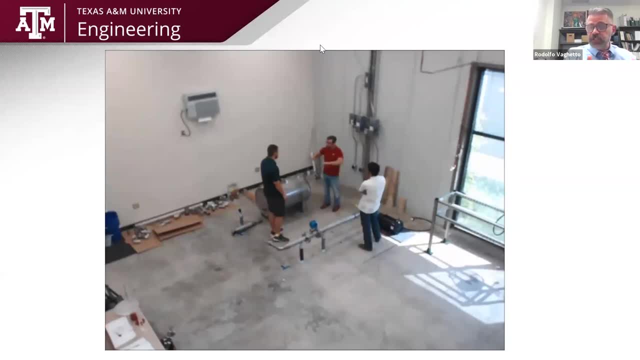 depending on the type of spacing technology, but this is not in principle an issue, because there are other attachments at the bottom and top of the core that prevented the fuel assembly from moving Right, But the entire – that wire wrap doesn't put a – like a – like a – as neutral. 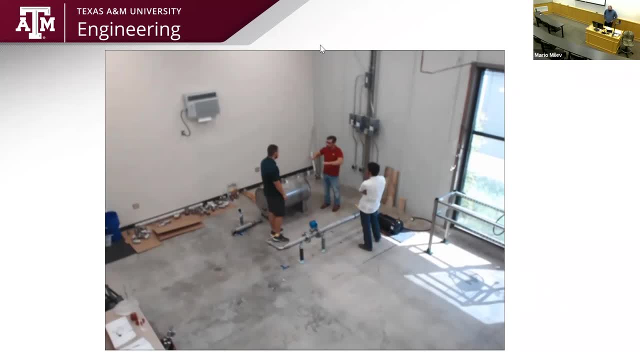 torque on it. I mean it starts to – I mean imagine it's – I mean imagine it's – it's like twisting those things or something. Well, that – and that's –, for example, if you look at the pressure distribution, that 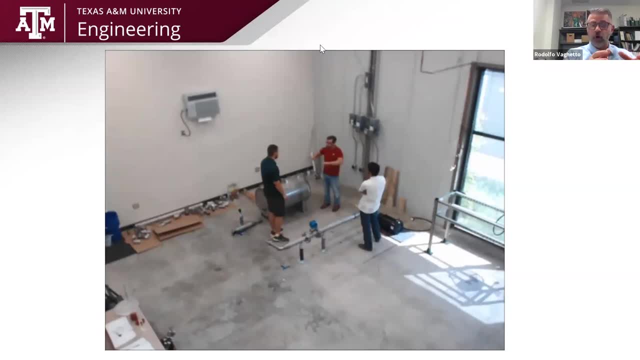 I mentioned. that is very important. So the – the pressure forces that you – that you develop by the fact that this wire will create like a – a transverse flow. it's actually important to know, because it may create the flow – a spin, displacement, or. 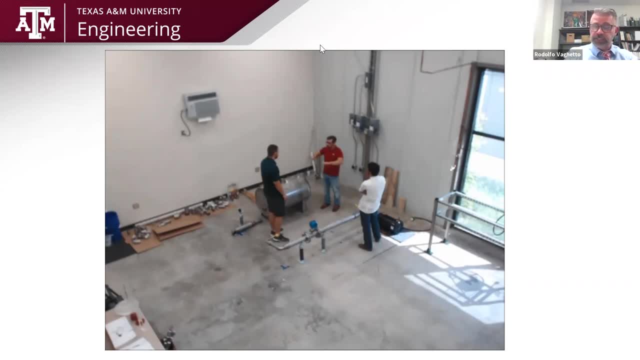 it has an impact on the flow-induced vibration. So these are – these are the reason why we are – we are conducting this experiment. This is the major difference from – for example, of a light-water reactor, where you don't have these radial forces induced by. 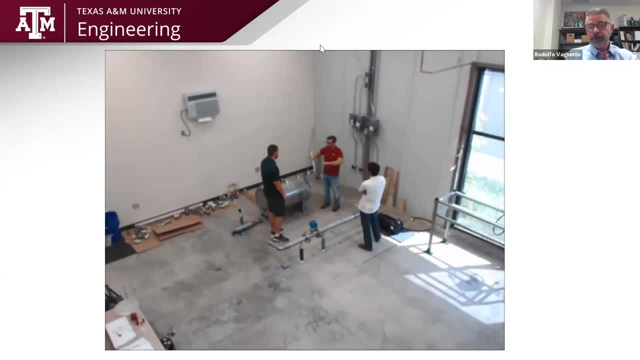 the – by the wire in this case. Thank you. So we have one question on the chat from Chen-Kai Tai, who asks: – Sure, Are there any special? – are there any special treatments to overcome the optical opaqueness of liquid metal, so that PIV-like technique could be applied in liquid metal experiments? 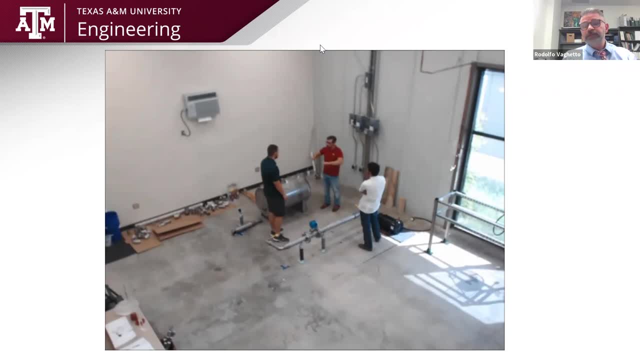 Well, that is a good question. As a matter of fact, I would say: if you in the future know of any way to apply a PIV technique in liquid metal, I will be more than happy to know. But you cannot apply flow this way. 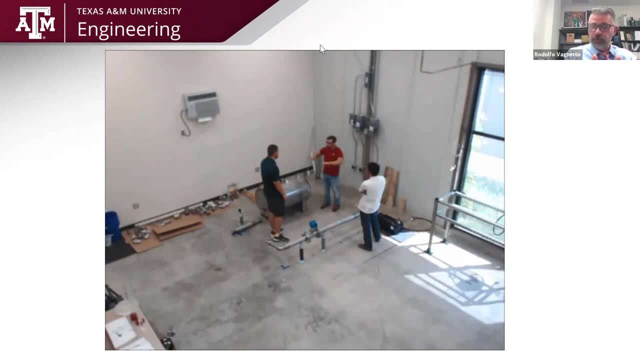 Okay, You can use the special qualification technique in the strict term of the – of the definition because, again, by definition, you need to have a transparent fluid And in fact that's why all these tests that we have conducted, we have conducted with surrogate fluid. So 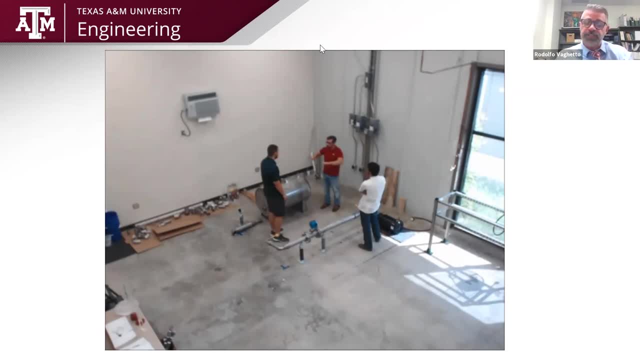 now, if you use a surrogate fluid, you can match a certain property, and with proper scaling. Now, if you do a hydraulic test, so isotherapy, you can match a certain property, So isothermal tests, like I mentioned. you care about the Reynolds number? 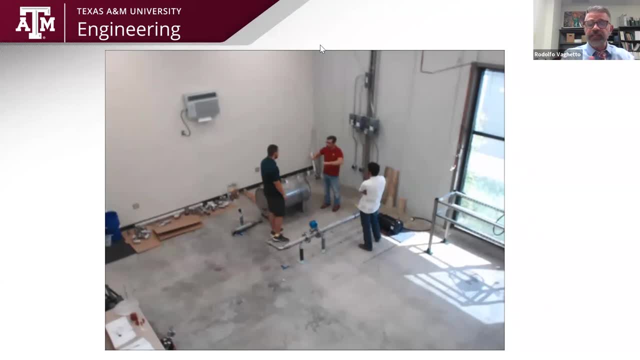 So, as long as you match the Reynolds number, all these techniques are available and the results you obtain are directly transferable to your final configuration, which is liquid metal. There are other techniques. if you mean PIV-like, you mean, for example, techniques that will give you more high-resolution measurements. then there are some techniques for liquid metal, like ultrasonic techniques. 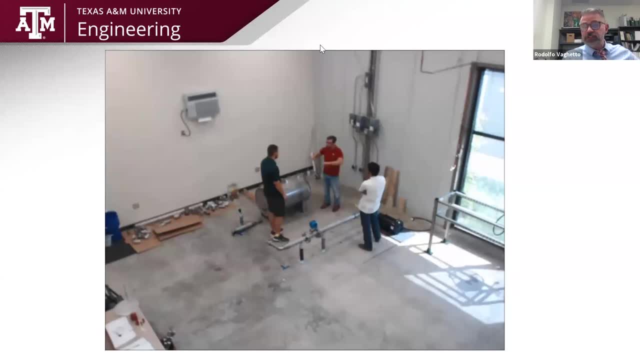 These are non-invasive techniques that may give you the ability to measure the flow in very small regions. So there are some other techniques that you can do. So there are some other techniques that you can do. In our experimental test campaign, we have chosen to use a surrogate. Subsequently, we were able to directly deploy the PIV in our bundle. 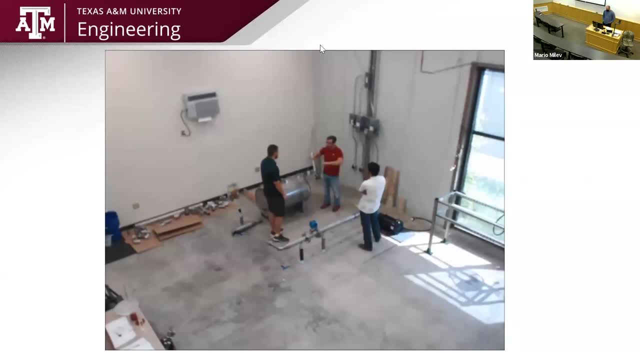 Thank you, Okay, any other questions from our audience? Last chance for the semester After this. you got to wait till after Christmas to ask questions. So what are the non-nuclear engineering applications that was mentioned that they are made in dialogue? 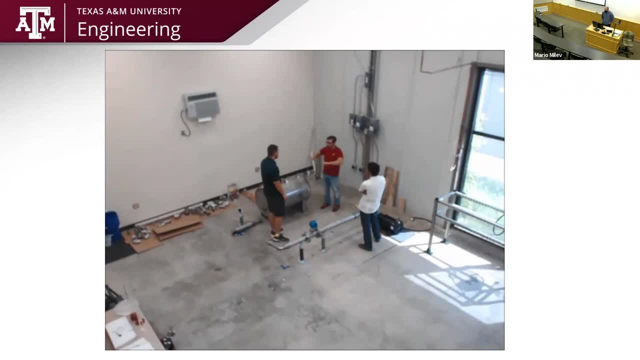 Say that again. You mentioned that you also do some non-nuclear engineering applications or measurements. So non-nuclear applications, Yeah, So I believe I recognize the voice of Dr Avramova, but I didn't actually hear the question. 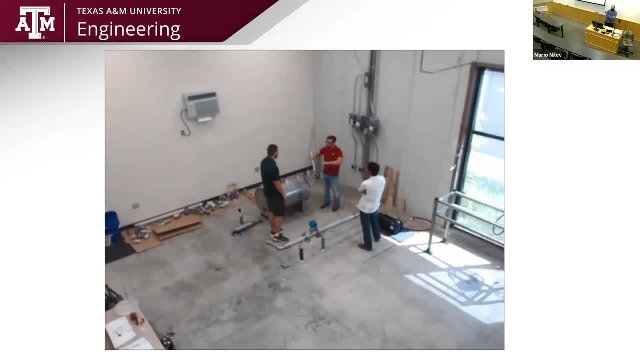 So she was curious about Some of the non-nuclear applications that you work on in your lab. Well, so molten salts we are studying Molten salts are used for applications that are not as a coolant in the nuclear reactor. 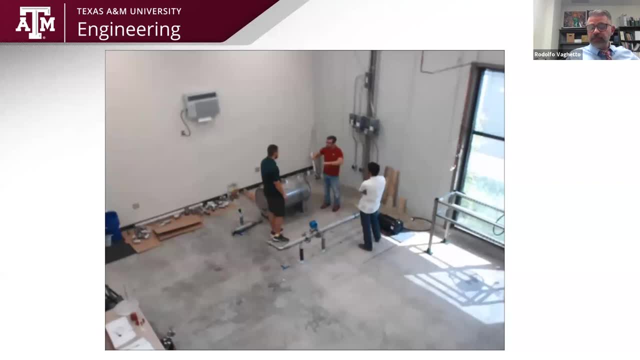 They are used as energy storages. So the same type of measurements that we have developed we are trying to deploy in molten salt for energy storage. Okay, We have done tests for two-phase that are not directly related to the nuclear industry. 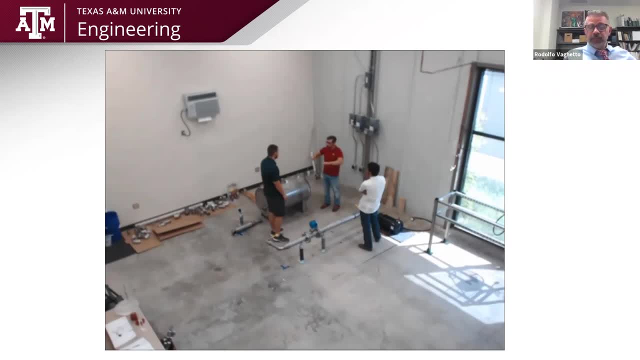 So there are really certain activities that we are trying to deploy for non-nuclear applications. There are some space applications we are also working on right now where you can imagine all these techniques are available and can be easily deployed. So we have another question on the chat. 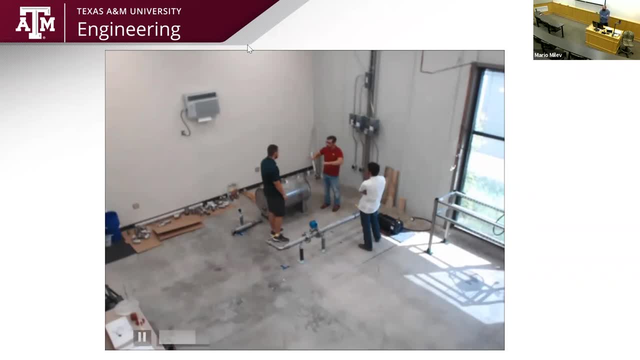 Joy Fan asks: with MIR method in a turbulent study, will the uncertainty increase in the thin boundary layer since the walls are not visible anymore? Well, the measurement near the wall and very like within the boundary layer- So we are talking in the extreme vicinity of the wall- are very challenging. 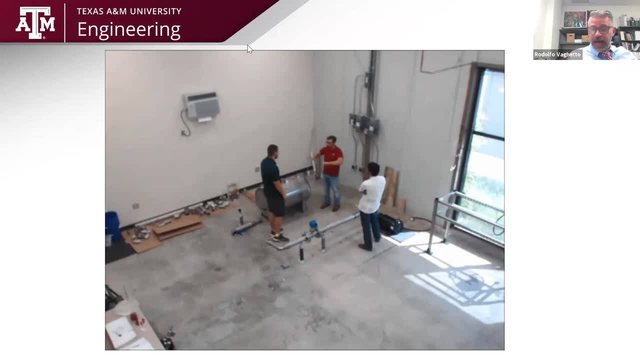 And everything depends on the light, the illumination, the calibration you are doing near the wall. So there is not a direct answer. In principle, the MIR method works, But it's the combination of your light source and the ability to see the 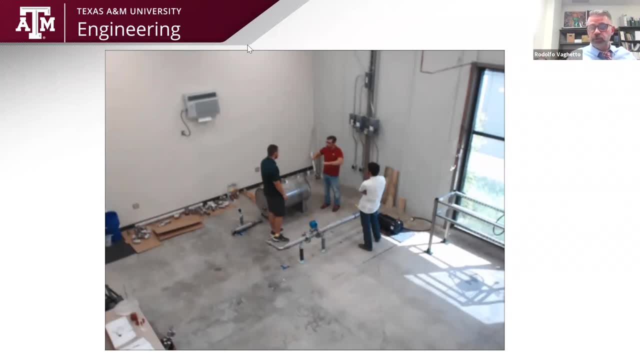 the particles near the wall without any other disturbance, and most likely is the reflection from the wall. That is what causes you to increase the uncertainty at the point that you really need not to consider your experimental data near the wall. And this is an answer that you will have depending on your geometry, depending on your setup, depending on your flow conditions as well. 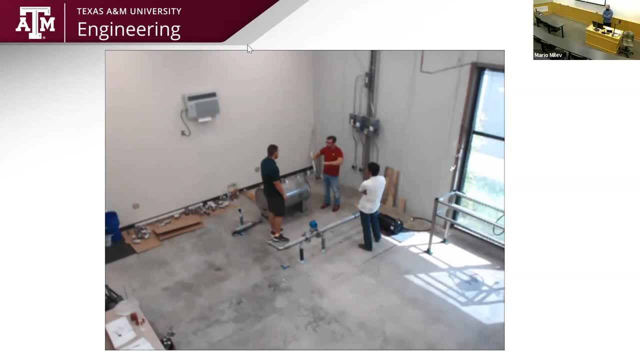 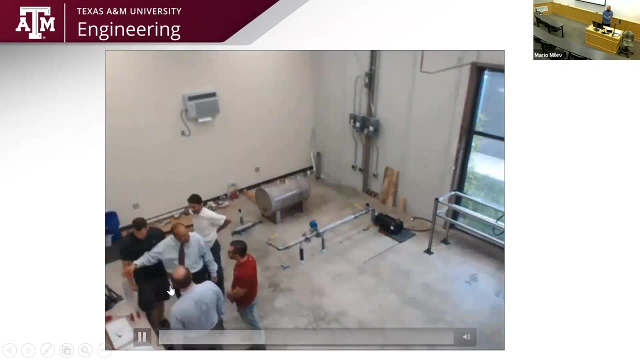 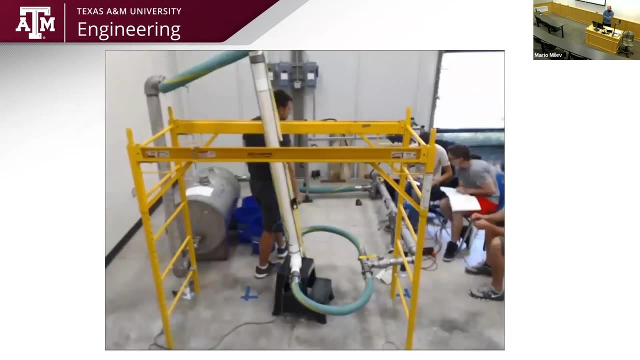 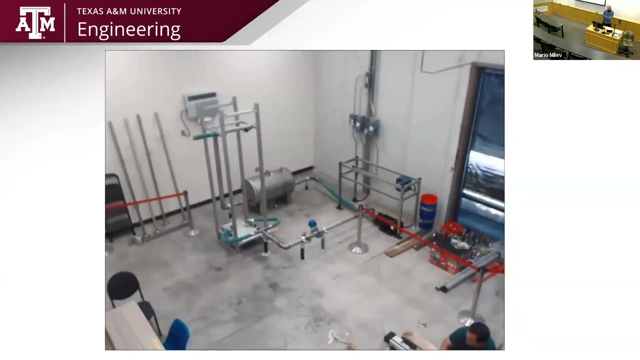 Thank you. I mean, could you put up This might be a silly question, Could you? just? You still have the matched index of refraction, So you aren't getting the distortion of the laser light coming through the system. But could you use a fluid that has a dye in it so that, even though you aren't getting distortion, you're still being able to differentiate between the wall location and the fluid? 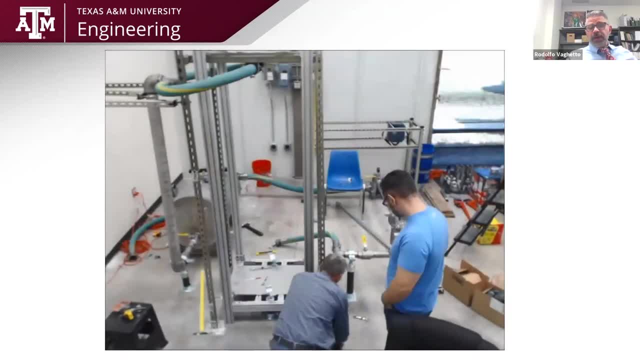 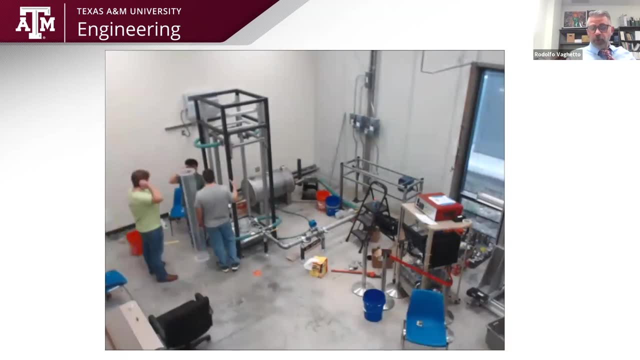 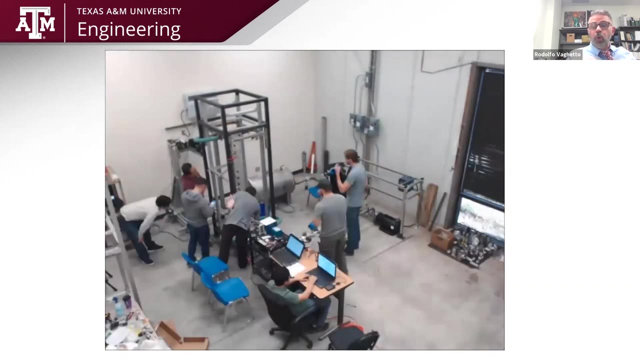 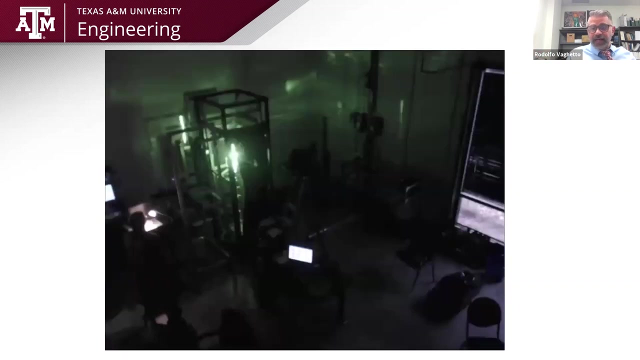 Would that help? Yeah, That's basically So. even if you have a matched index of refraction, the matching is never perfect And it's the ability of the experimentalist to quantify the uncertainty. So in the uncertainty quantification there is a step, that is the calibration, that allows you to estimate the distortion. 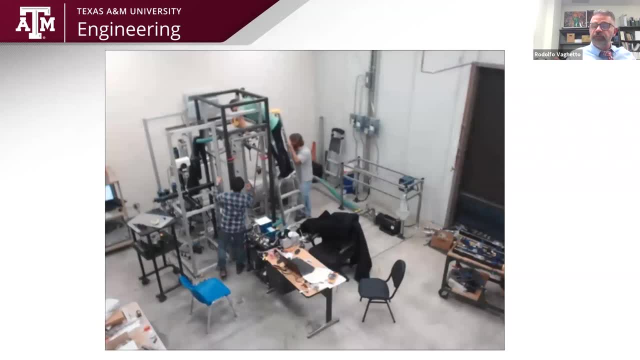 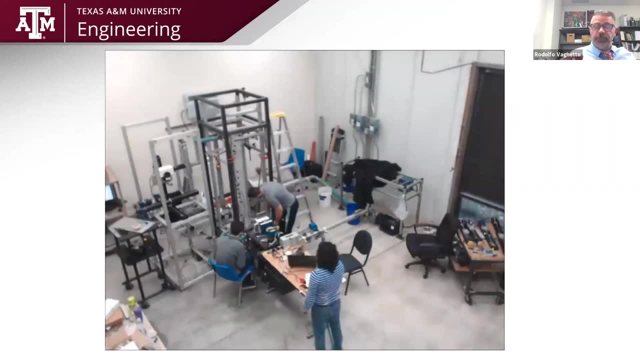 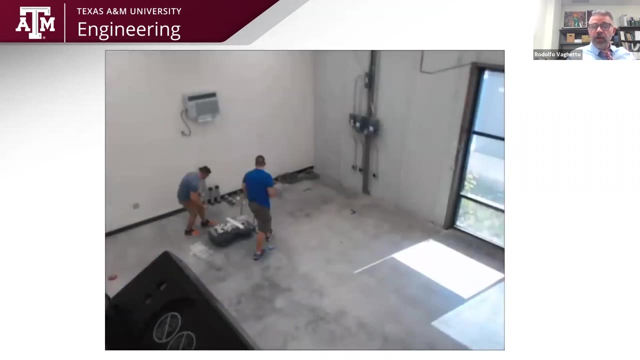 That you have for the presence of the walls, the solid walls, the liquid, the not perfect matching between the index of refraction and the walls. There is other type of research that you can do, for example, even further improve the matching between the liquid and the solid. 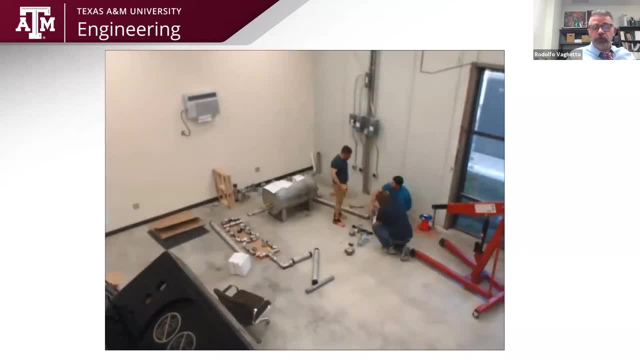 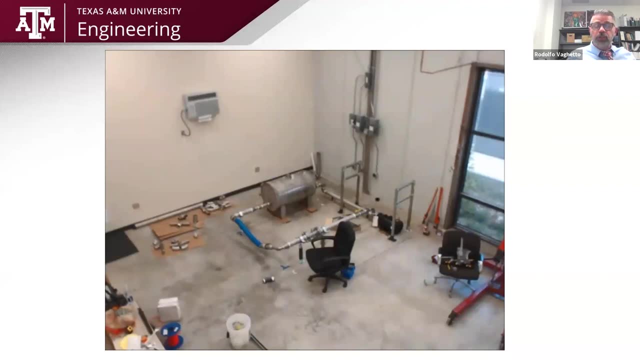 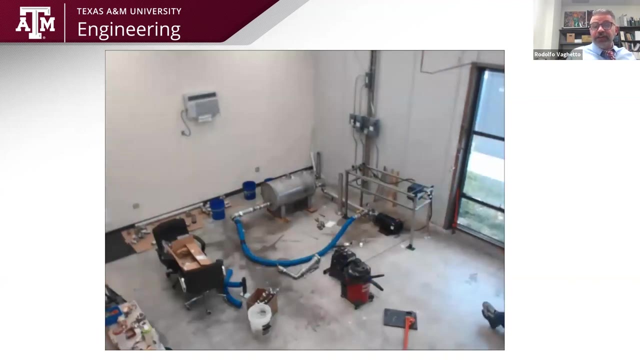 So this is one thing that we have done in our lab: Instead of using, let's say, the coupling Peace, I mean with the acrylic- We have explored the other material and liquid that can give you even better and even more limited distortion when you run the experiment. 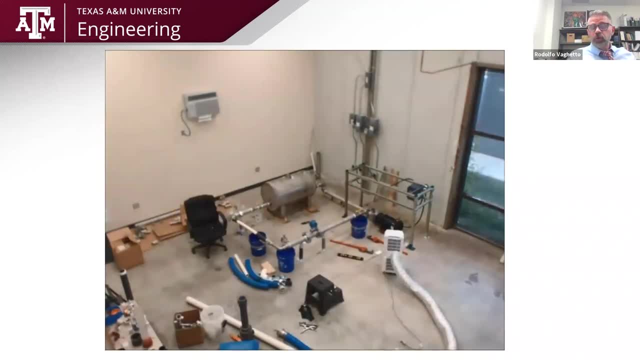 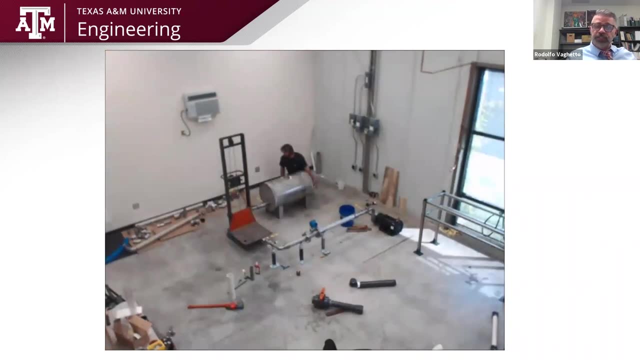 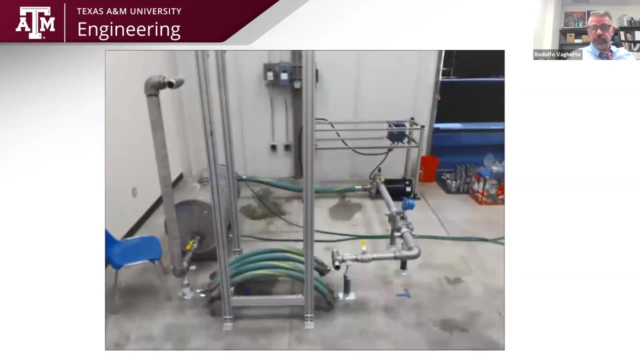 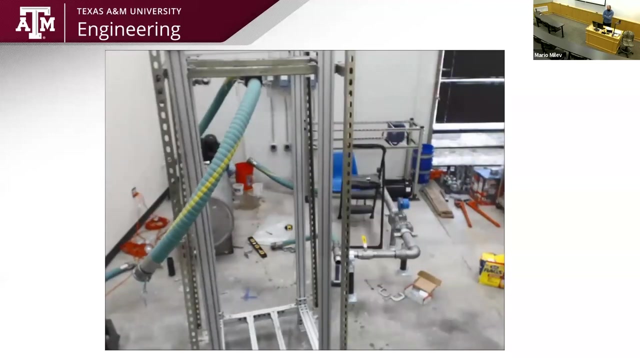 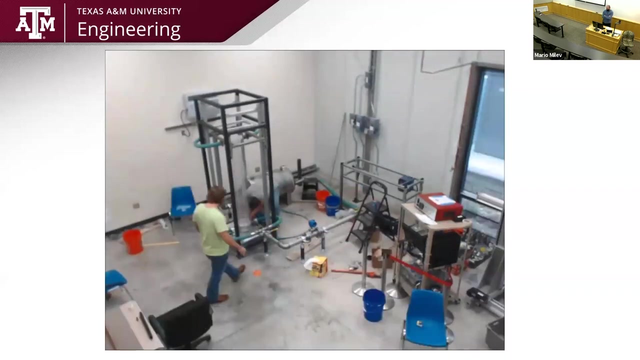 So you have two ways to work here. One is, quantify uncertainty- That is mandatory for any experiment- But second, try to minimize the distortion By using more sophisticated fluids and solids- clear material. I'm watching this time-lapse video and sometimes not now. I'll be really curious to hear what kind of safety nightmare it is having that laser light reflecting off of everything while people are in the room. 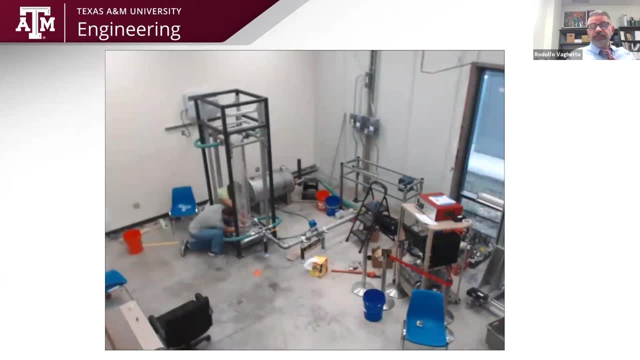 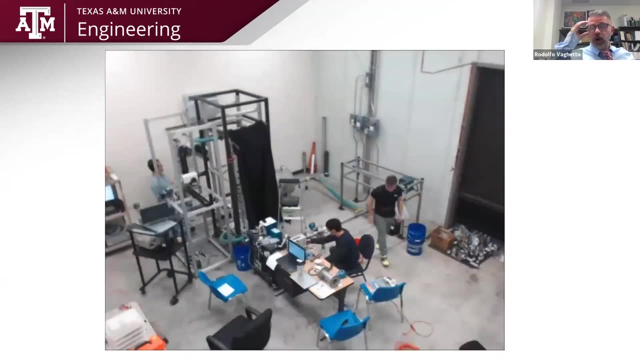 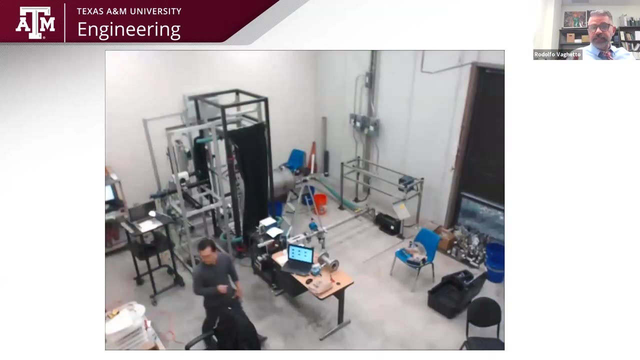 That's got to be. That must have been fun. Oh yeah, Well, in fact, this is a closed room And everyone using the laser You need to have the safety goggles on The safety goggles. basically what they do is they screen the laser at that specific wavelength. 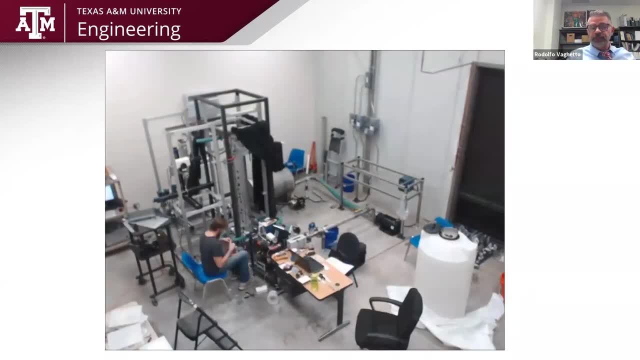 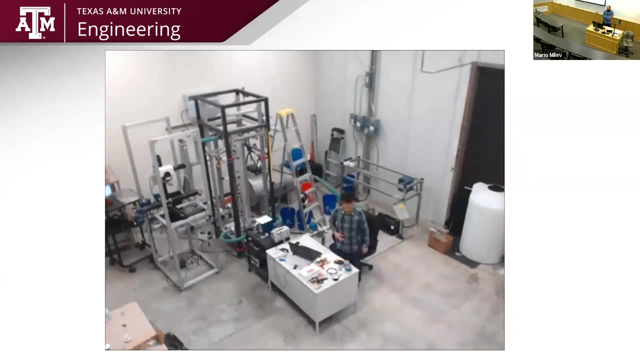 And that is the way you prevent and you maintain safety when running these experiments. Still, just, It's impressive. I mean, I'm pretty. I could just imagine our safety guy having a heart attack if he saw this. This is impressive. 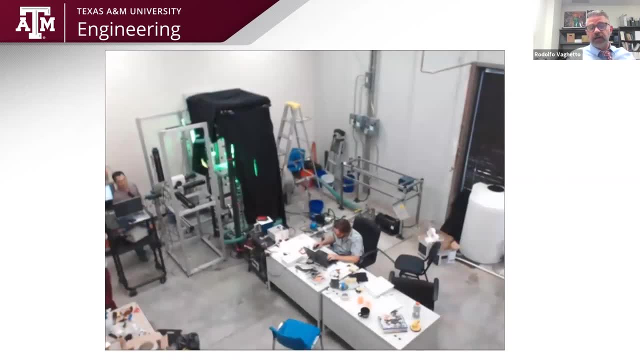 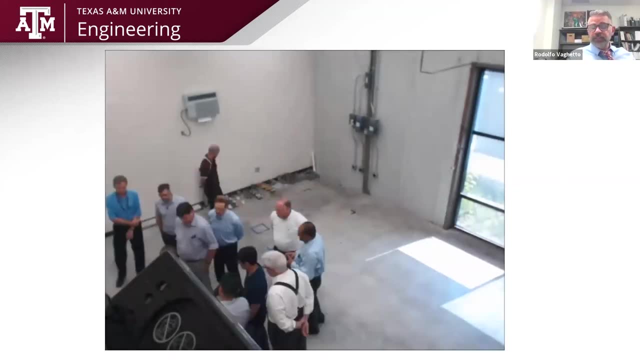 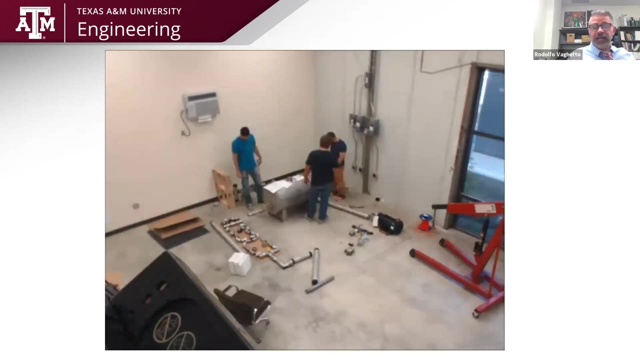 Oh yeah, Well, our safety guy. I have a safety guy too And that's a major problem. A major issue when you set up an experimental activity like this one is making sure there is an area that is under control. You have safety feature to turn off the laser when someone accidentally opened the curtains or opened the door. 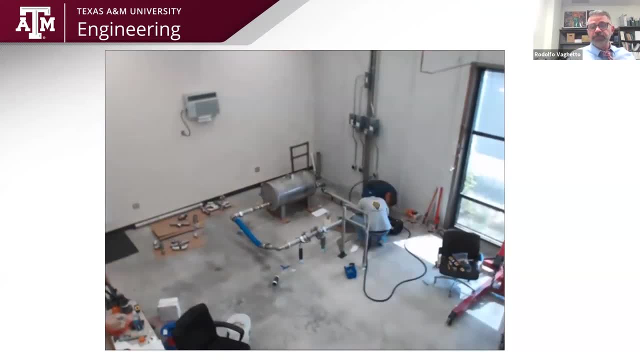 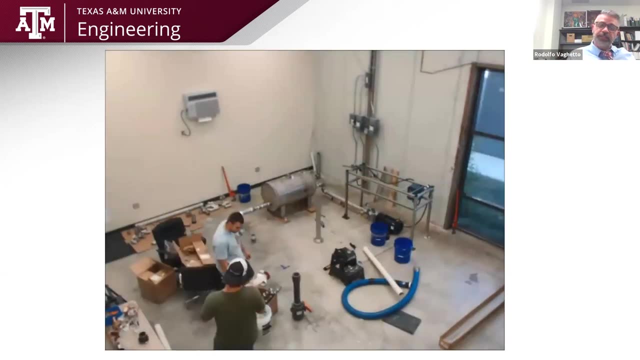 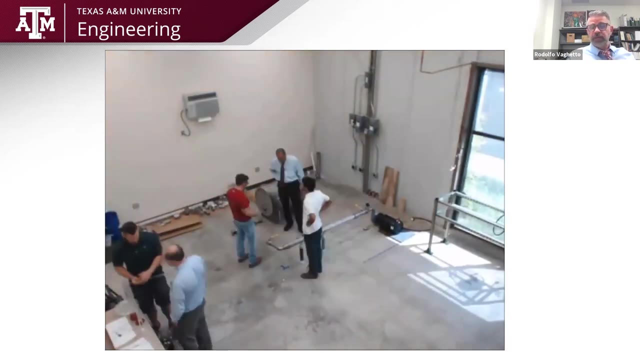 There are sound and light alarms that are everywhere in the laboratory And everyone, even the ones that are not allowed to use the laser, they need to take the laser separately. They need to take the laser separately- training, because they need to know how to cooperate with the experimental activity going on in the lab. 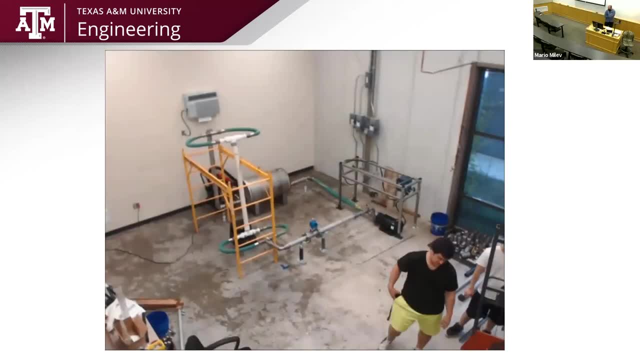 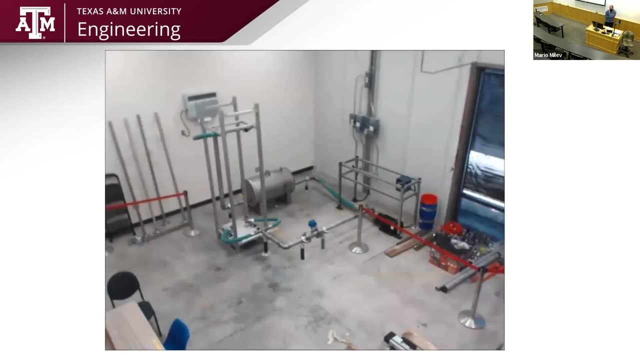 Okay, One more quick question, since they're not. What kind of laser is it? What kind of power is it? Is it just a Just a yak with a? It looks like a yak with a. Yeah, It's a green laser. 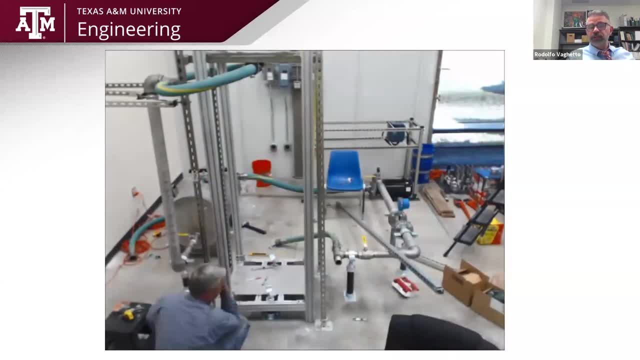 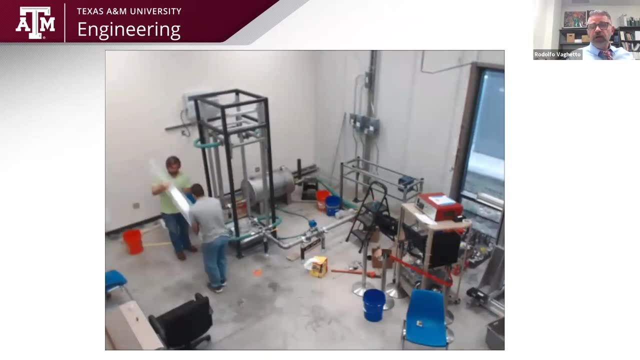 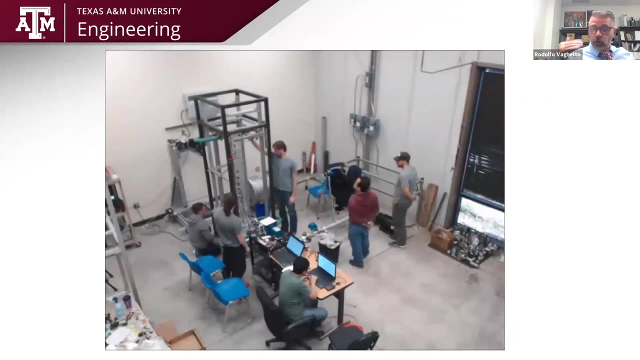 The wavelength is 530 nanometer. The power: It usually depends on the penetration that you need to achieve. We range from 10, 20 power laser. This is a pulse laser, But we have also continuous lasers that we use for other applications. 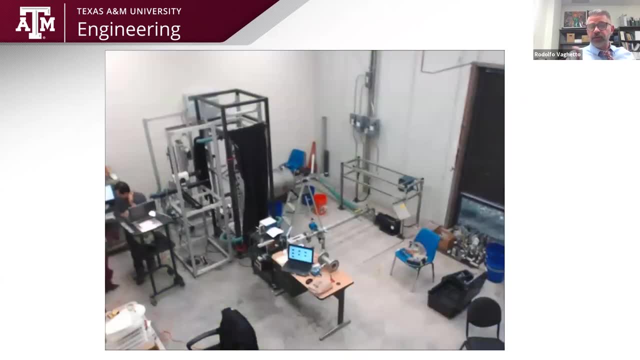 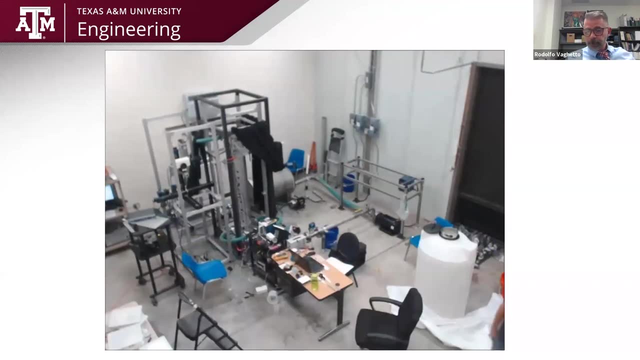 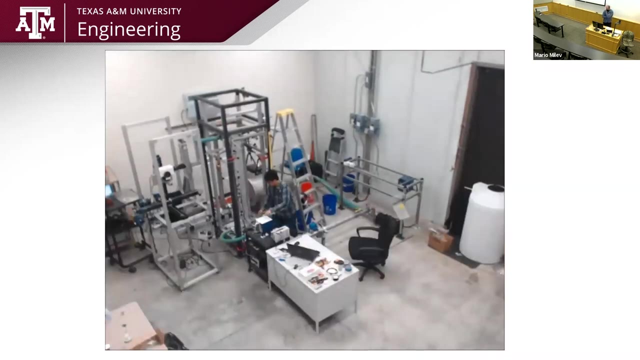 So most of our laser is in the range of 530 nanometer. We have other lasers that we use for other applications- Great, Okay, Well, if there's not any other questions, I guess we're going to go ahead and close out this session. 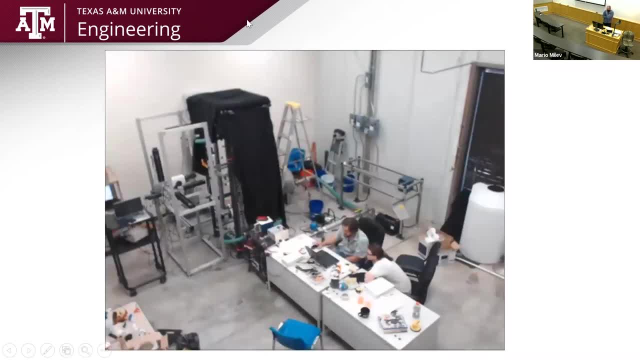 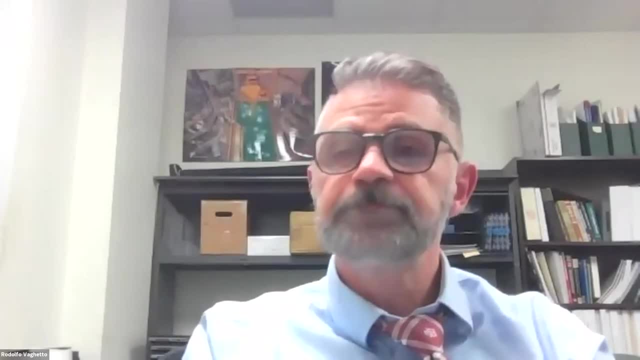 Special thanks to our speaker for a great presentation. I appreciate it. Thank you And thanks to everyone for participating. Thank you for inviting and thank you everyone for staying here. Have a great holiday, Eat lots of turkey and see you in the new year. 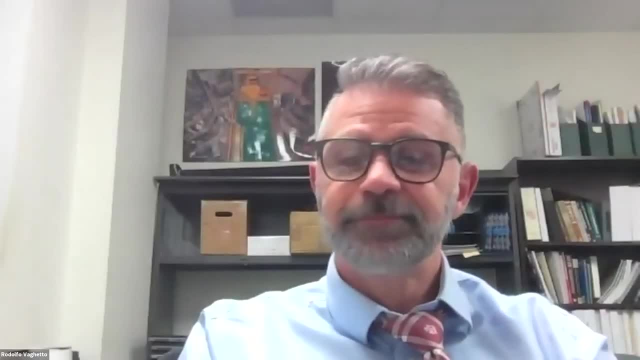